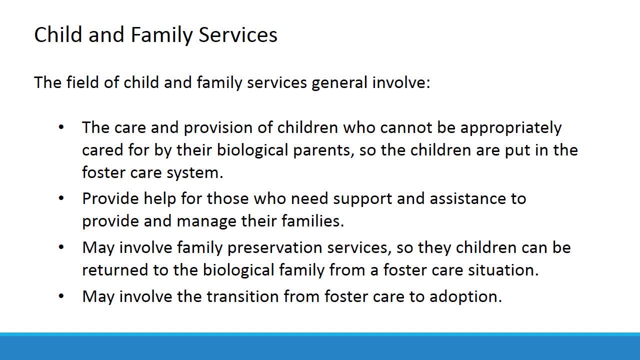 They provide help for those who need support and assistance to provide and manage their families, and may involve family preservation services so the children can be returned to the biological family from a foster care situation. It may also involve the transition from foster care to adoption. 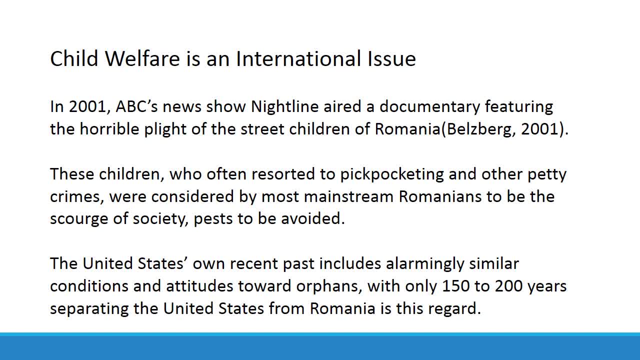 Child welfare is an international issue. In 2001, ABC's news show Nightline aired an article about child welfare. It was aired a documentary featuring the horrible plight of the street children of Romania. These children are often resorted to pickpocketing and other petty crimes are considered by most mainstream Romanians to be the scourge of society. pests to be avoided. 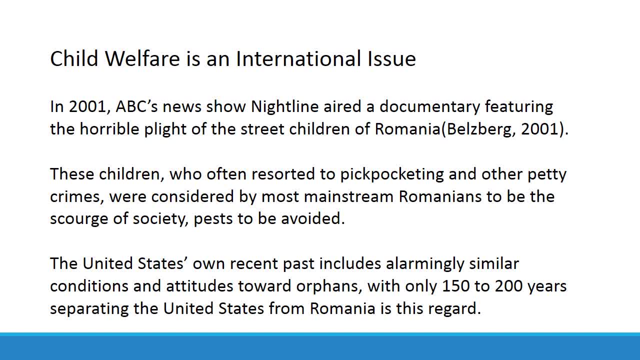 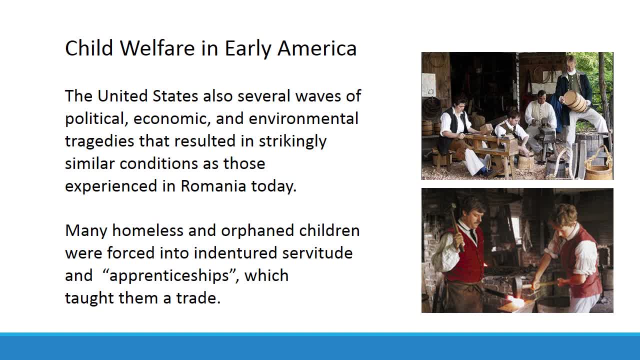 The United States own recent past includes alarmingly similar conditions and attitudes towards orphans, with only 150,000.. The United States own recent past includes alarmingly similar conditions and attitudes towards orphans, with only 150,000.. United States also had several waves of political, economic and environmental tragedies that 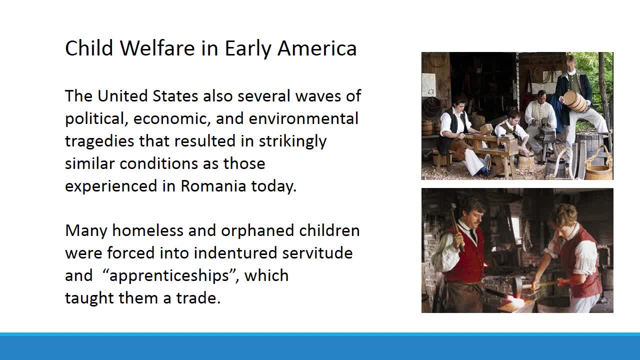 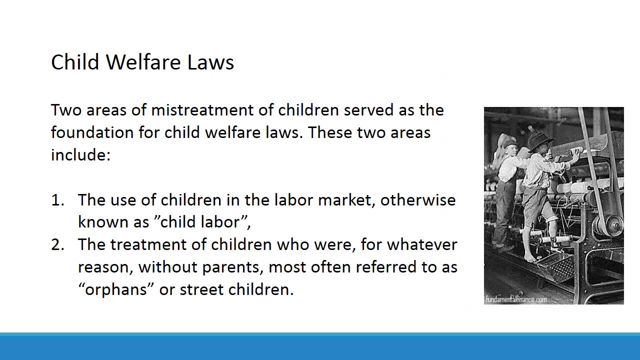 resulted in strikingly similar conditions as those experienced in Romania today. Many homeless and orphaned children were forced into indentured servitude and apprenticeships which taught them a trade- Two areas of mistreatment of children served as the foundation for child welfare laws. 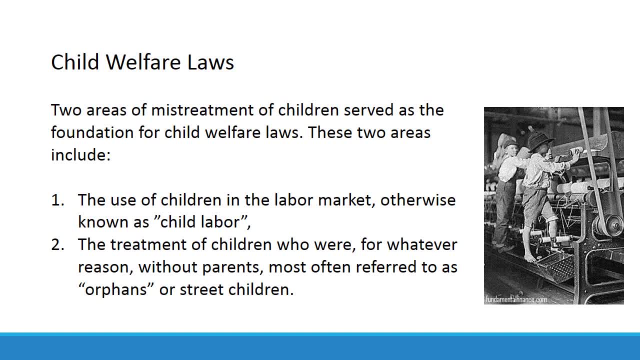 These two areas include: 1. The use of children in the labor market, otherwise known as child labor. You'll see on the right hand side a picture from the late 1800s, early 1900s, where you see young children, clearly no older than 9 or 10 years old, working textile machines. 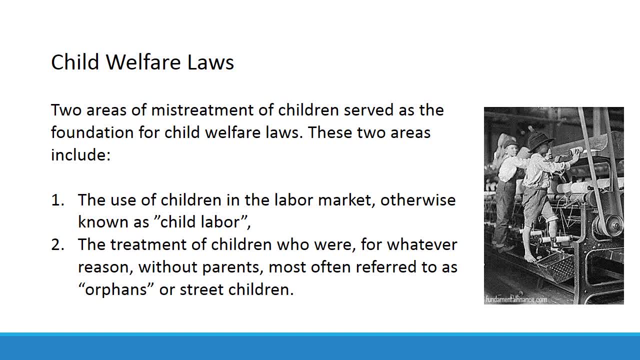 2. The treatment of children who were, for whatever reason, without parents, most often referred to as orphans or street children. 3. The treatment of children who were, for whatever reason, without parents, most often referred to as orphans or street children. 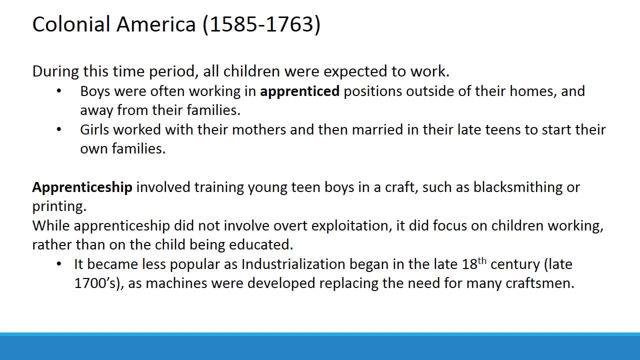 4. The treatment of children who were, for whatever reason, without parents, most often referred to as orphans or street children. So let's start and go back to colonial America, which, for most historical purposes, runs from about 1585 to 1763.. 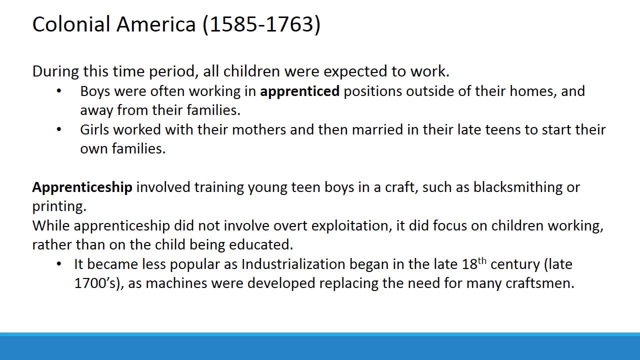 During this time period, all children were expected to work. Boys were often working in apprenticed positions outside of their homes and away from their families. Girls worked with their mothers and then married in their families, their late teens, to start their own families. Apprenticeship involved training young teen. 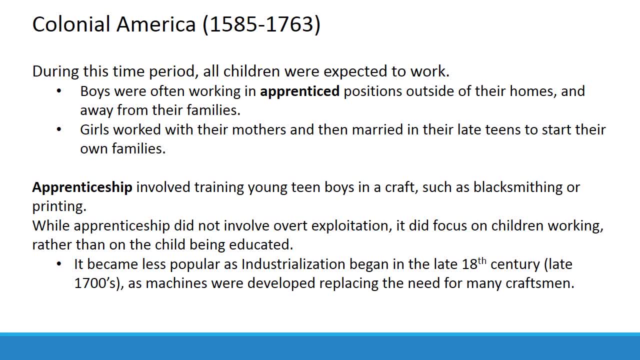 boys in a craft such as blacksmithing or printing. While apprenticeship did not involve overt exploitation, it did focus on children working rather than on the child being educated. It became less popular as industrialization began in the late 18th century or the late 1700s. 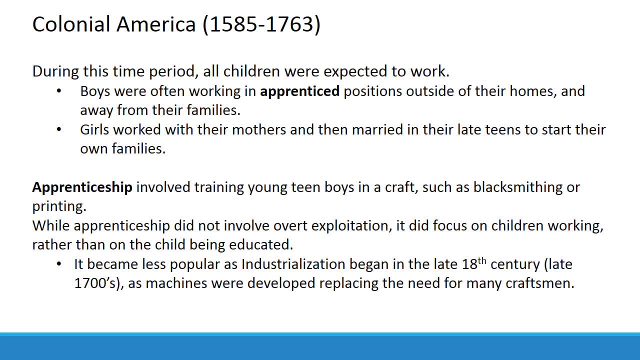 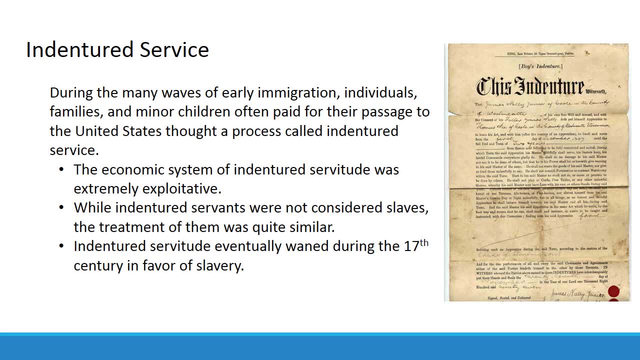 as machines were developed, replacing the need for many craftsmen. During the many waves of early immigration, individuals, families and minor children often paid for their passage to the United States through a process called indentured service. The economic system of indentured servitude was extremely exploitive, While indentured servants 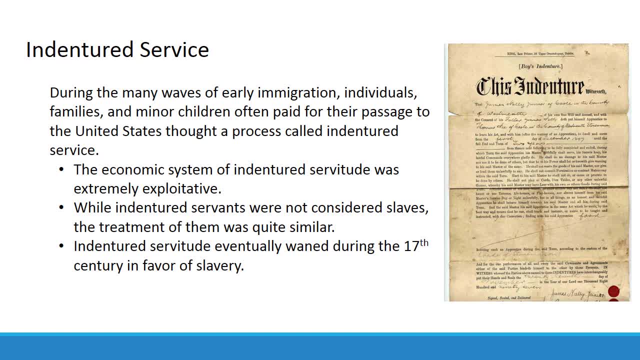 were not quite indentured. they were not quite indentured. Inventors were not considered slaves. Their treatment was quite similar. Indentured servitude eventually waned during the 17th century or the 1600s in favor of slavery. 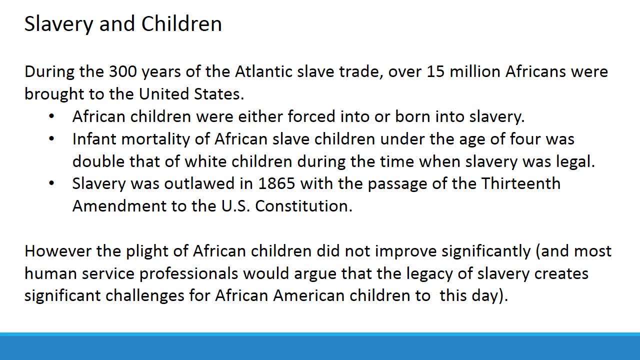 During the 300 years of the Atlantic slave trade, over 15 million Africans were brought to the United States. African children were either forced into or born into slavery. Infant mortality of African slave children under the age of four was double that of white children during the 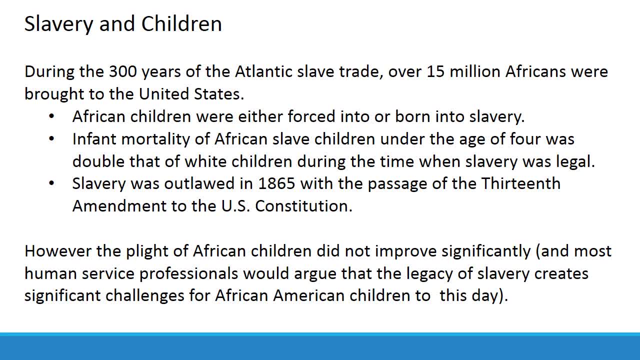 same time, during the time when slavery was legal, And just to kind of put that in context, you know we already have high mortality rates in this era, but the mortality rates for African slave children were double, absolutely double, that of white children. 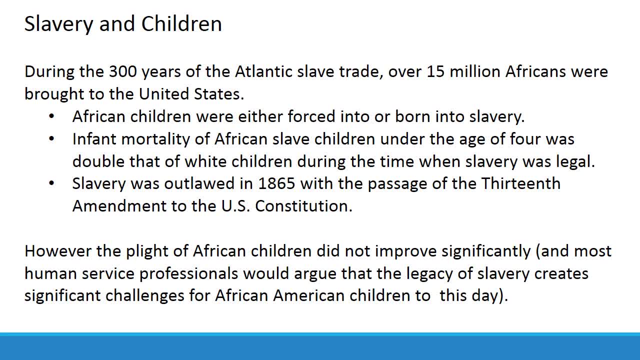 Slavery was outlawed in 1865 with the passage of the 13th Amendment to the US Constitution. However, the plight of African children did not improve significantly, and most human service professionals would argue that the legacy of slavery creates significant challenges for African American children to this day. 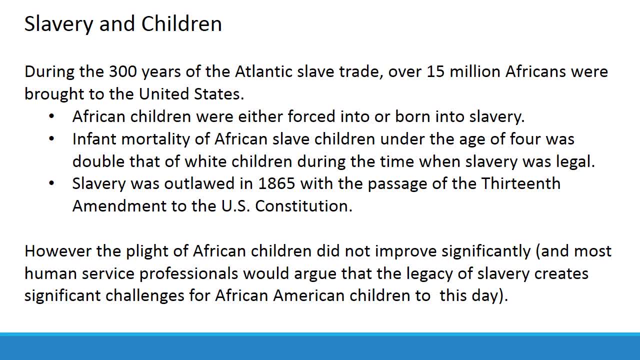 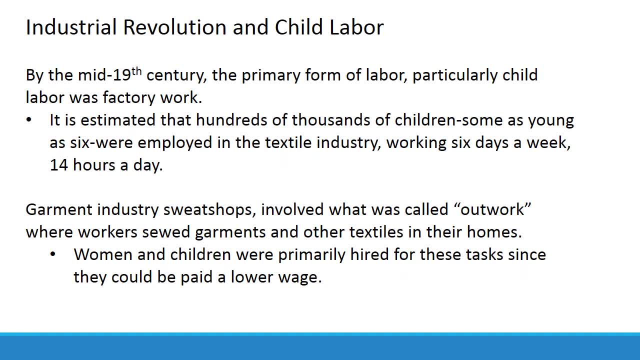 There's a lot of institutional racism and in a variety of classes you will see this addressed in a variety of ways. By the mid-19th century, the primary form of labor, particularly child labor, was factory work. It is estimated that hundreds of thousands of children, some as young as six, were employed in the textile industry, working six days a week, 14 hours a day. 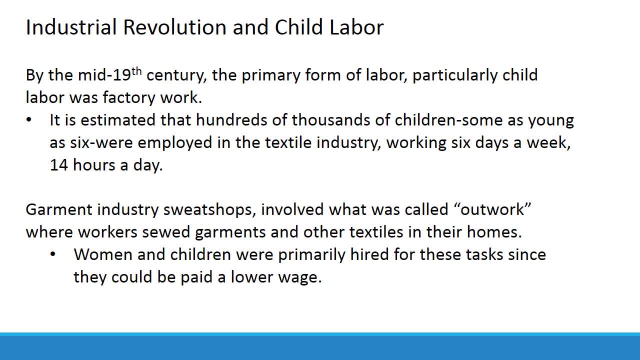 The labor market was a very important part of the labor market. The labor market was a very important part of the labor market. Garment industry sweatshops involved what was called outwork, where workers sewed garments and other textiles from their own homes. 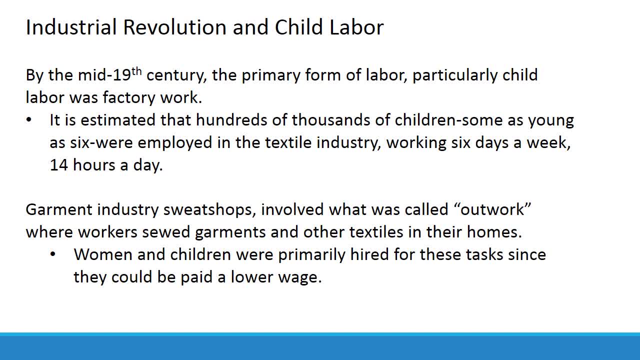 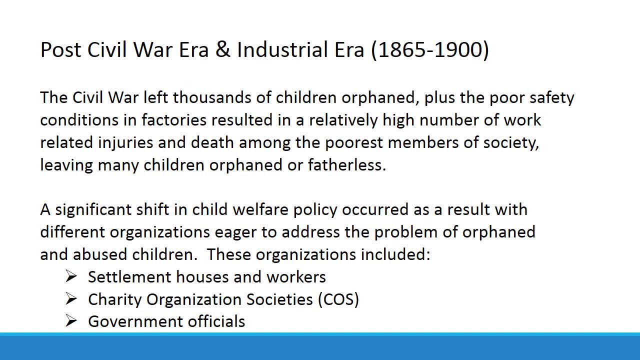 Women and children were primarily hired for these tasks, since they could be paid a lower wage. Post-Civil War era and the Industrial Era, which encompasses 1865 to 1900,. the Civil War left thousands of children orphaned. Plus, the poor safety conditions in factories resulted in relatively high number of work-related injuries and death among the poorest members of society. 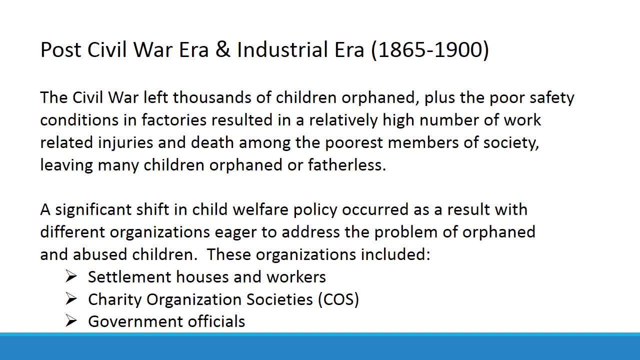 leaving many children orphaned or fatherless. A significant shift in welfare policy for children occurred as a result, with different organizations eager to address the problem of orphaned and abused children. These organizations included Settlement House Settlement Houses and Workers, as we've discussed with Jane Addams and Hull House. 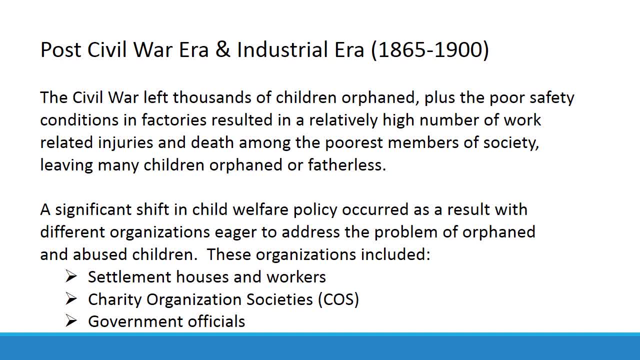 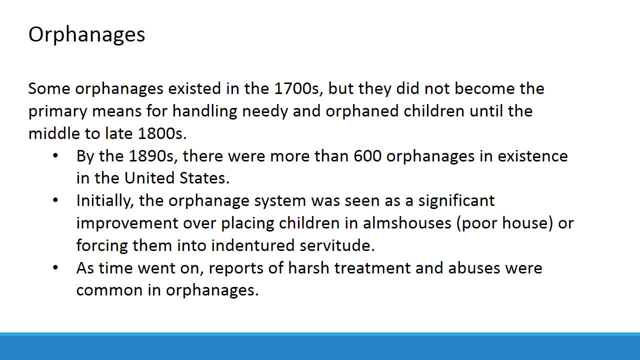 Charity Organization, Societies and Government Officials. Some orphanages existed in the 1700s, but they did not become the primary means for handling needy and orphaned children until the middle to late 1800s. By the 1890s there were more than 600 orphanages in existence. 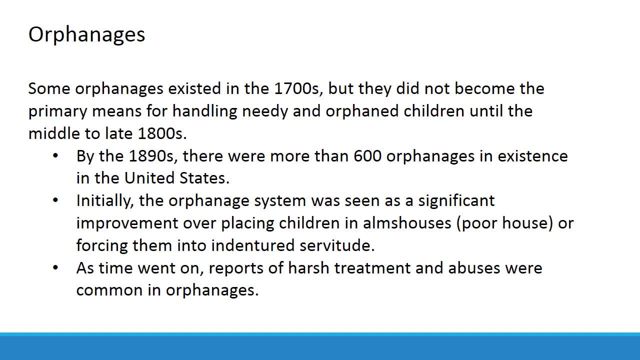 These organizations were also listed as the top five orphanage systems in the United States. Initially, the orphanage system was seen as a significant improvement over placing children in almshouses or poor houses or forcing them into indentured servitude. As time went on, reports of harsh treatment and abuses were common in orphanages. 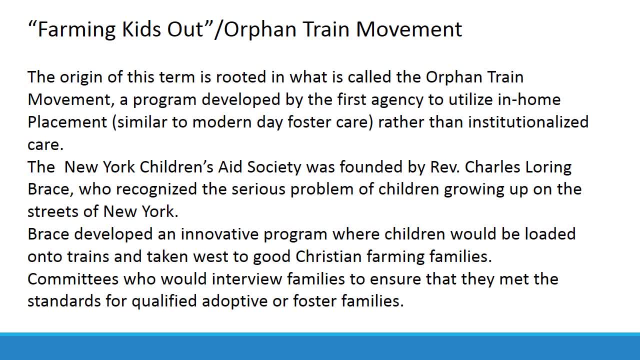 Then there became the orphan train movement or the term farming kids out. the origin of the name in our country, Something that had not yet been used to begin the name yet. The origin of a grade 10 child听. The origin of a grade 10 child tongue: tongue-telling. 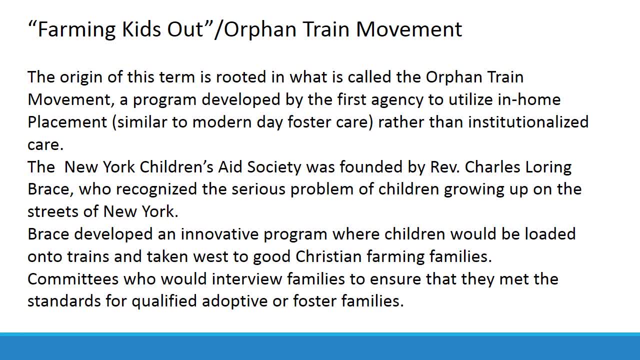 this term is rooted in what is called the Orphan Train Movement, a program developed by the first agency to utilize in-home placement, which is similar to modern day foster care, rather than the institutionalized care model of having children all live in an orphanage. The New York Children's 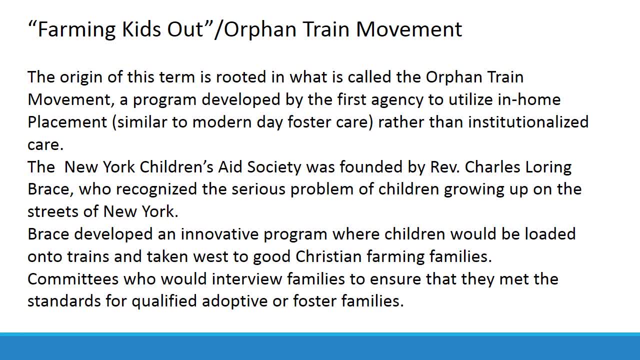 Aid Society was founded by the very reverend Charles Loring Brace, who recognized the serious problem of children growing up on the streets of New York. Brace developed an innovative program where children would be loaded onto trains and taken west to good Christian farming families. 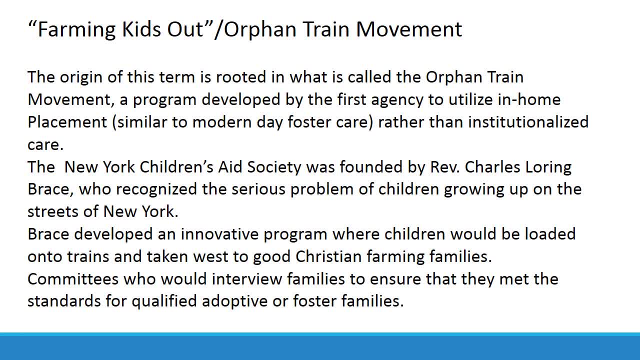 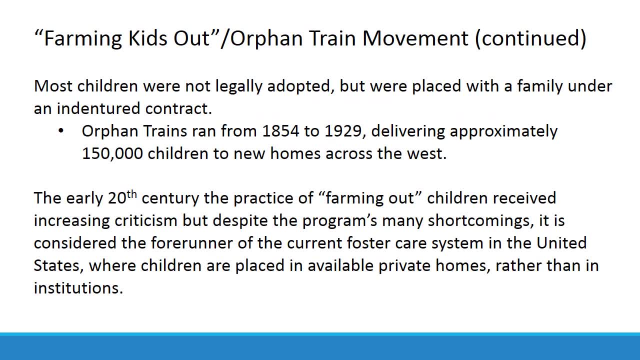 committees, who would interview families to ensure that they met the standards for qualified adoptive or foster families. Most children were not legally adopted but were placed with a family under an indentured contract. Orphan trains ran from 1854 to 1929, delivering approximately 150,000 children to new homes across. 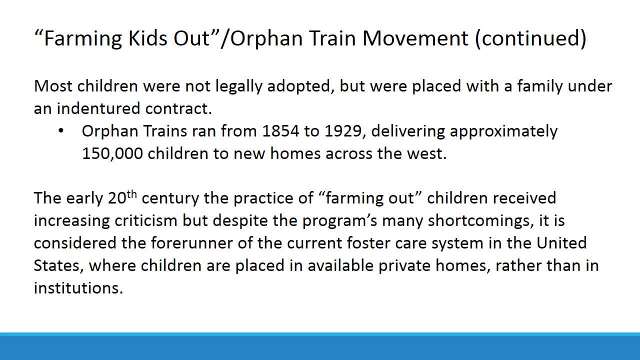 the West, The early 20th century, the practice of farming out children received increasing criticism. but despite the program's many shortcomings, it is considered the forerunner of the current foster care system in the United States, where children are placed in available. 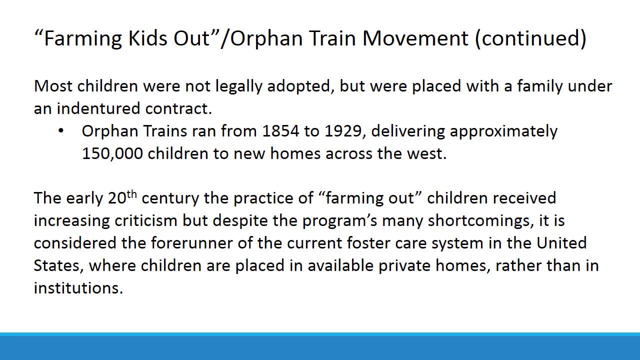 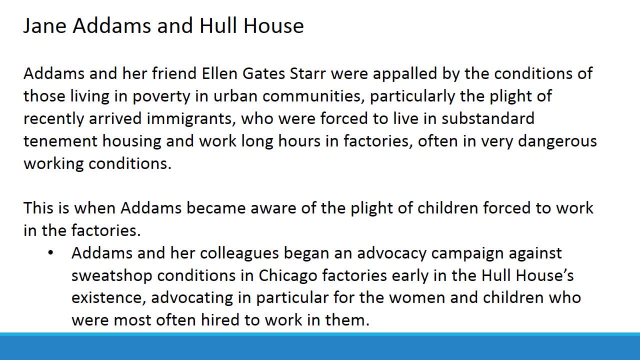 private homes rather than in institutions. Jane Adams and her friend Ellen Gates Starr were appalled by the conditions of those living in poverty in urban communities, particularly the plight of recently arrived immigrants who were forced to live in substandard tenement housing and work long hours. 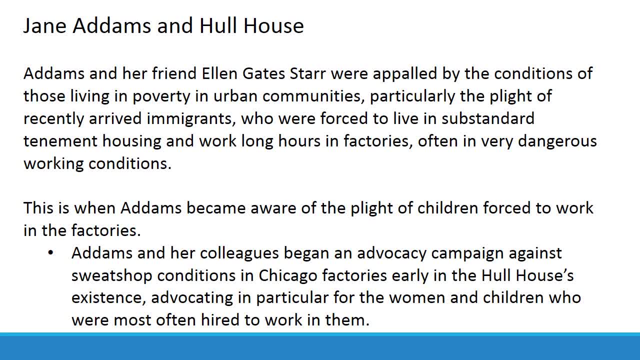 in factories, often in very dangerous working conditions. This is when Adams became aware of the of children forced to work in the factories. Adams and her colleagues began an advocacy campaign against sweatshop conditions in Chicago factories early in the Hull House's existence, advocating in particular for the women and children who were most often hired to work in them. 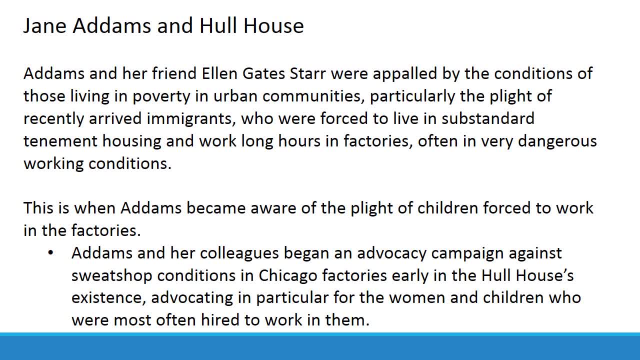 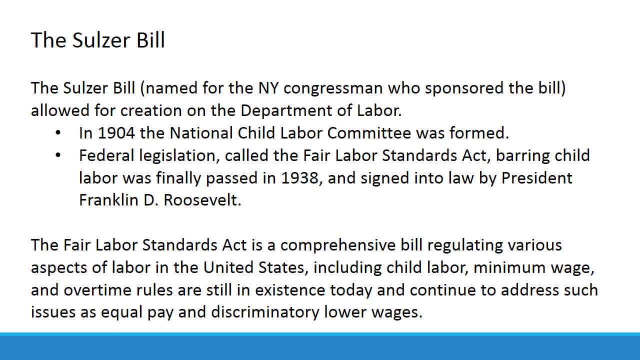 And again, Hull House was a settlement house that Jane Adams created. The Sulzer Bill, which was named for the New York congressman who sponsored the bill, allowed for the creation of the Department of Labor In 1904, the National Child Labor Committee. 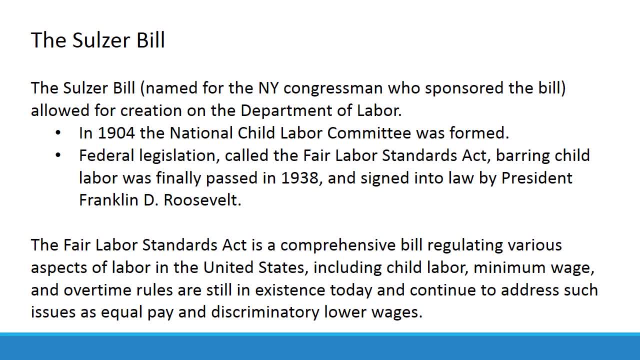 was formed, and federal legislation called the Fair Labor Standards Act barring child labor was finally passed in 1938 and signed into law by President Franklin D Roosevelt. The Fair Labor Standards Act was passed in 1934, and the National Child Labor Committee was formed in 1934. 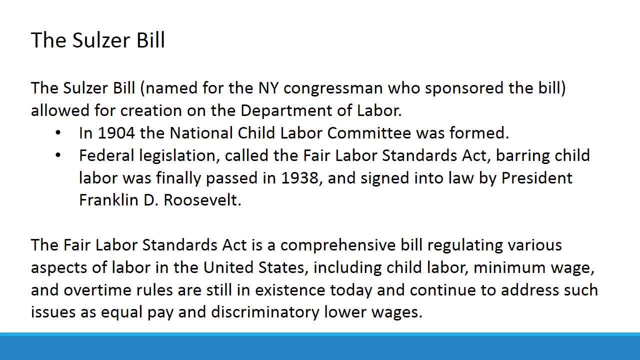 The Fair Labor Standards Act is a comprehensive bill regulating various aspects of labor in the United States, including child labor, minimum wage and overtime rules, which are still in existence today and continue to address such issues as equal pay and discriminatory lower wages. 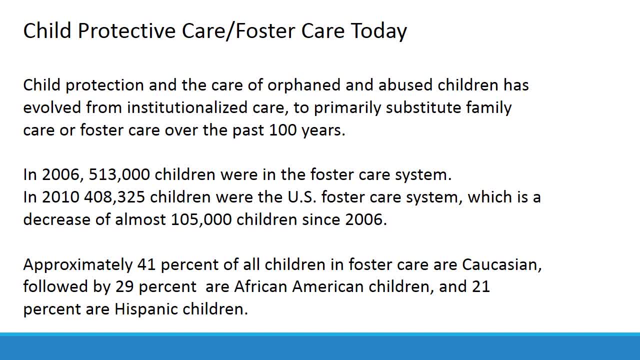 So let's look at the child protective foster care system today. Child protection and the care of orphaned and abused children has evolved. from the 19th century to the present. The child protection system has evolved from institutionalized care or orphanages to primarily substitute family care. 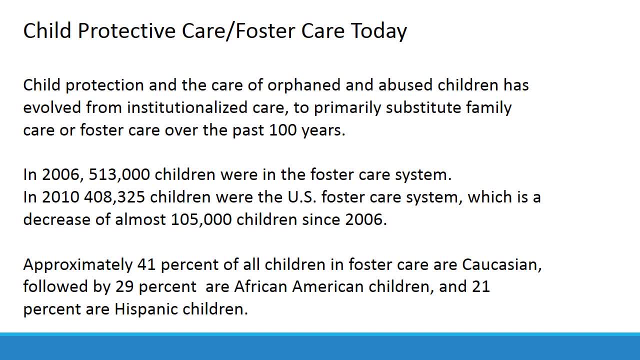 or foster care over the past 100 years. In 2006,, over a half a million children were in the foster care system. By 2010,, that number had decreased to 408,000 children, Almost 100,000, over 100,000. 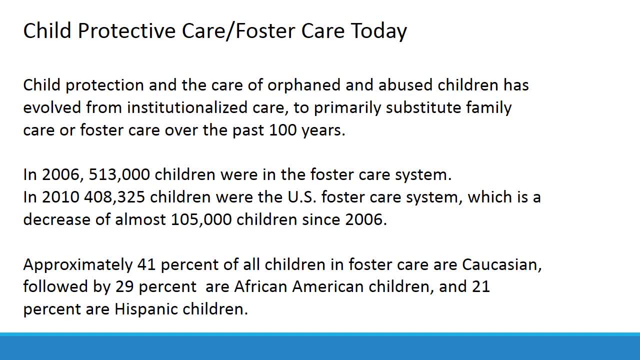 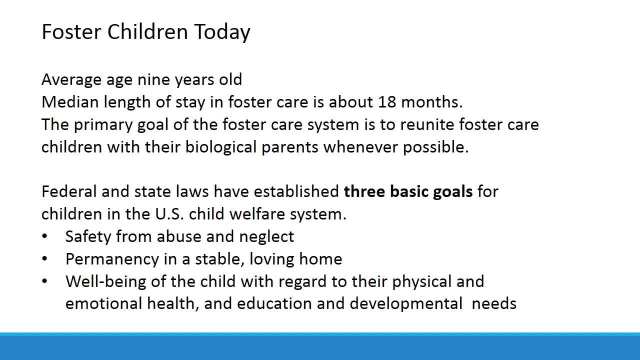 children had fallen from the system. Approximately, the number of children in the foster care system has increased by over 100,000.. Approximately 41% of all children in foster care are Caucasian, 29% are African American and 21% are Hispanic. The average age of a foster child is 9 years old. 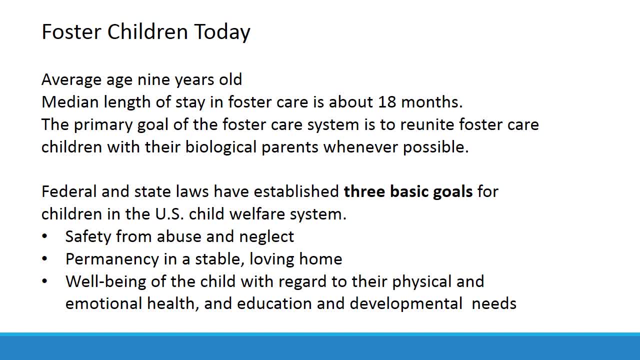 The median length of stay is about 18 months and the primary goal of the foster care system is to reunite foster care children with their biological parents whenever possible. Federal and state laws have established three basic goals for children in the United States child welfare system. One: safety from abuse and neglect. Two: permanency in a stable 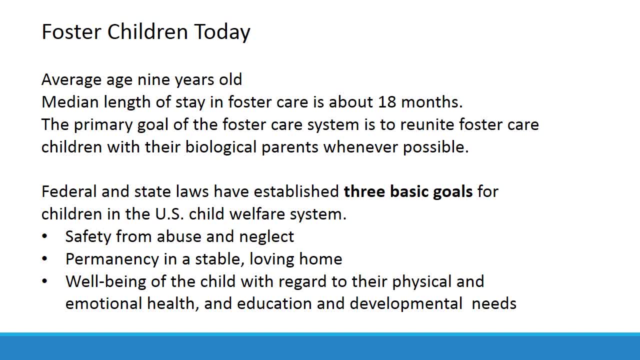 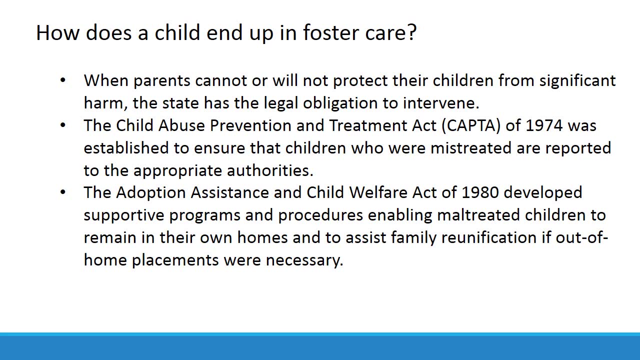 loving home. Three: well-being of the child with regard to their physical and emotional health, and education and developmental needs. So How Does a Child End Up in Foster Care? When parents cannot or will not protect their children from significant harm, the State has the legal obligation to intervene. The 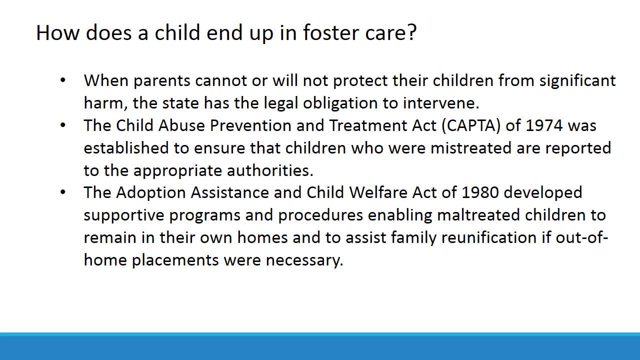 Child Abuse Prevention and Treatment Act of 1974 was established to ensure that children who are mistreated are reported to the appropriate authorities. The Adoption, Assistance and Child Welfare Act of 1950 is the first act of the child welfare act in the United States. It 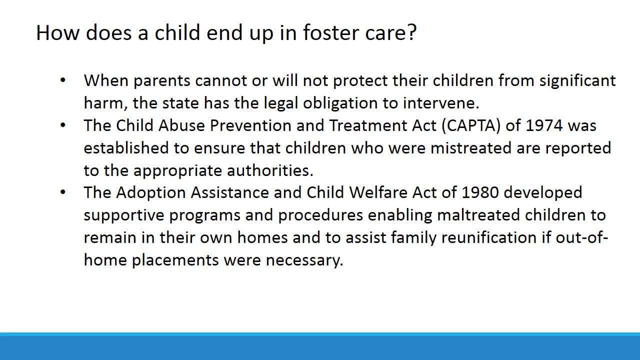 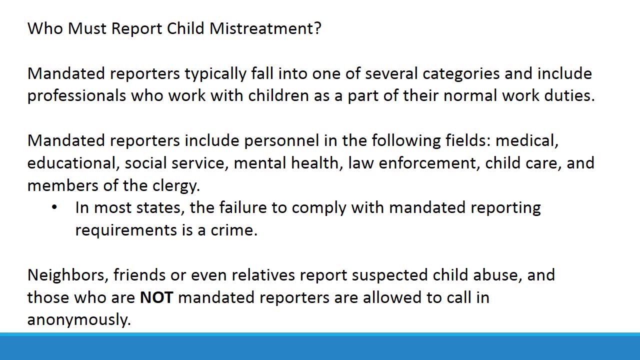 is the first act of the child welfare act of the United States. The adoption assistance develop supportive programs and procedures enabling maltreated children to remain in their own homes and to assist family reunification if out-of-home placements were necessary. Who must report child mistreatment? 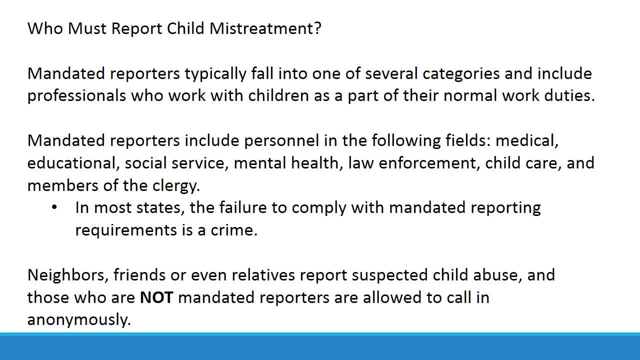 Mandated reporters typically fall into one of several categories and include professionals who work with children as part of their normal work duties. Mandated reporters include personnel in the following fields: medical education, social service, mental health, law enforcement, child care and members of the clergy. 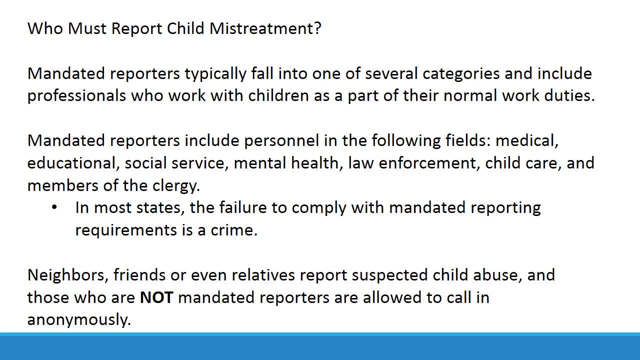 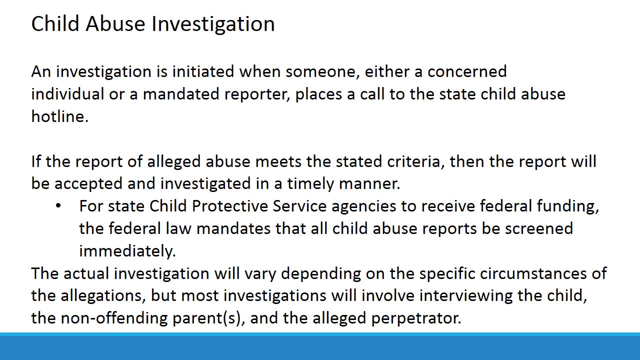 In most states, the failure to comply with mandated reporting requirements is a crime. Neighbors, friends or even relatives report suspected child abuse and those who are not mandated reporters are allowed to call it in anonymously. An investigation is initiated when someone, either a concerned individual or a mandated 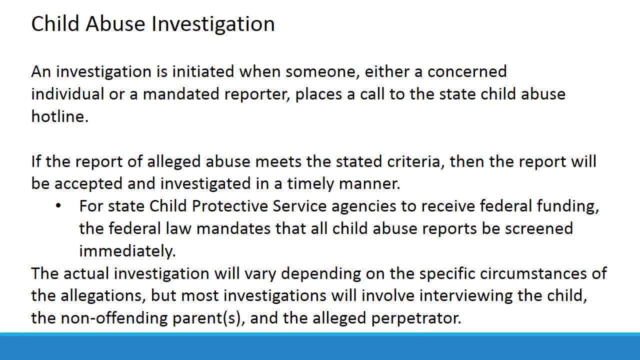 reporter places a call to the child state abuse hotline. If the report of an alleged abuse meets the stated criteria, then the report will be accepted and investigated in a timely manner. For state child protection, the report must be accepted and investigated in a timely manner. 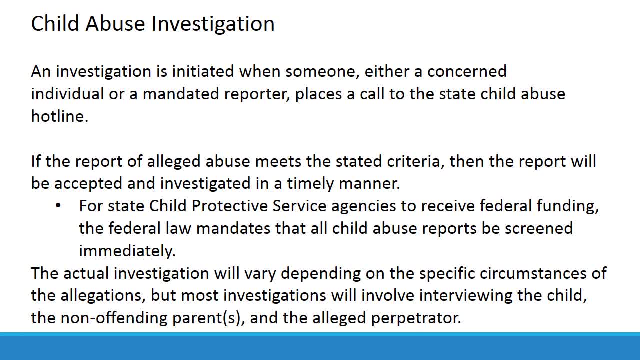 For state child protection. the report must be accepted and investigated in a timely manner To force protective service agencies to receive federal funding. the federal law mandates that all child abuse reports be screened immediately. The actual investigation will vary depending on the specific circumstances of the allegations. 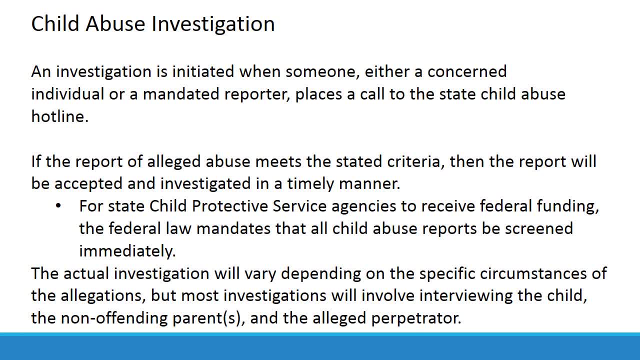 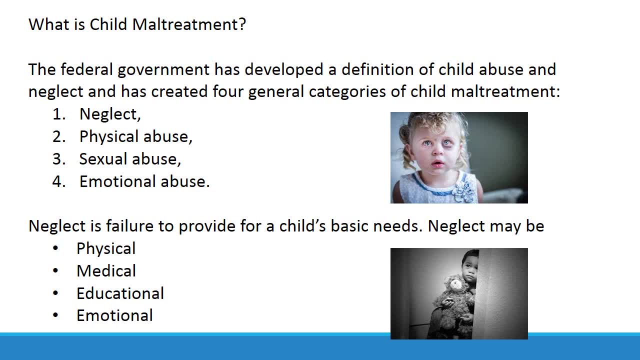 but most investigations will involve interviewing the child, the non-offending parent or parents and the alleged perpetrator. So What is child maltreatment? The federal government has developed a definition of child abuse and neglect and has created four general categories of child maltreatment. Number one: neglect. Number two: 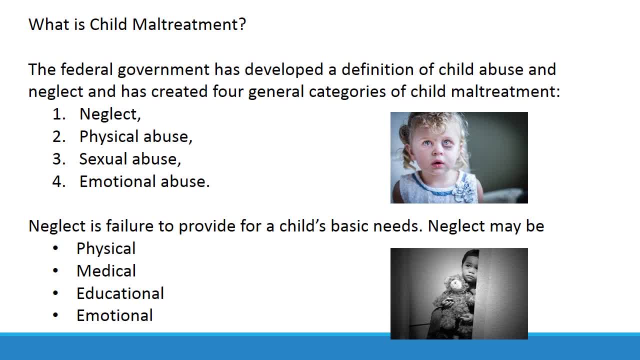 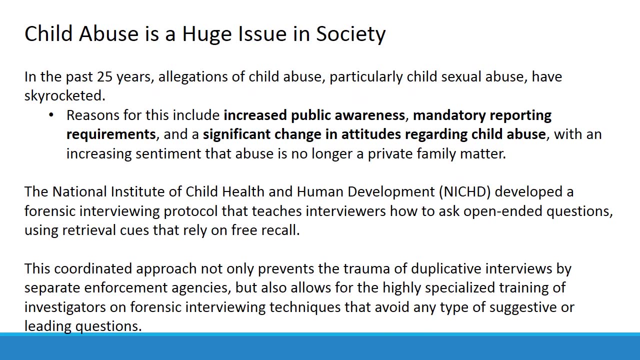 physical abuse. Number three: sexual abuse. Number four: emotional abuse. Neglect is failure to provide for a child's basic needs. Neglect may be physical, medical, educational or emotional. Child abuse is a huge issue in society. In the past 25 years, allegations of child abuse. 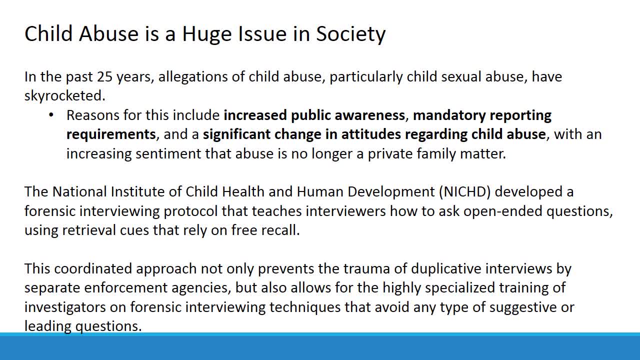 particularly child sexual abuse, have skyrocketed. Reasons for this include increased public awareness, mandatory reporting requirements and a significant change in attitudes regarding child abuse. with an increasing sentiment that abuse is no longer a private family matter, The National Institute of Child Health and Human Development developed a forensic 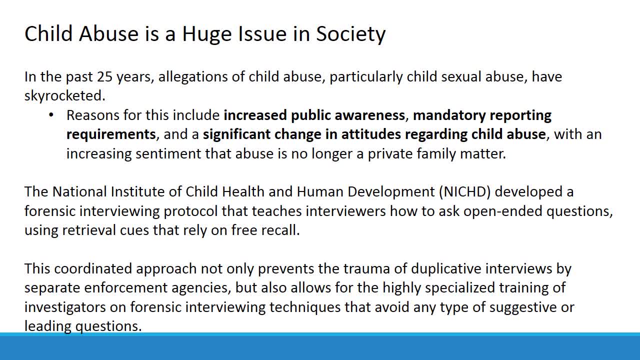 interviewing protocol that teaches interviewers how to ask open-ended questions using retrieval cues that rely on free recall. This coordinated approach not only prevents the trauma of duplicative interviews, but also prevents the trauma of duplicative interviews. The National Institute of Child Health and Human Development also allows for the highly specialized training of investigators. 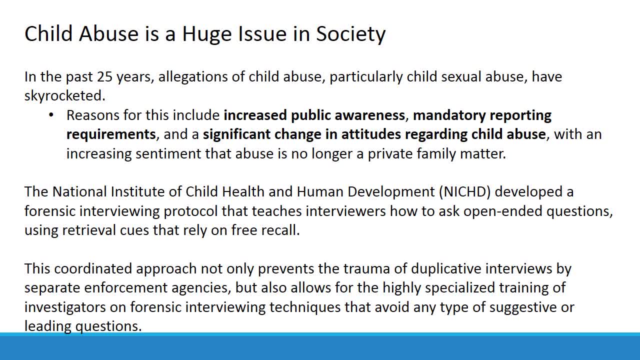 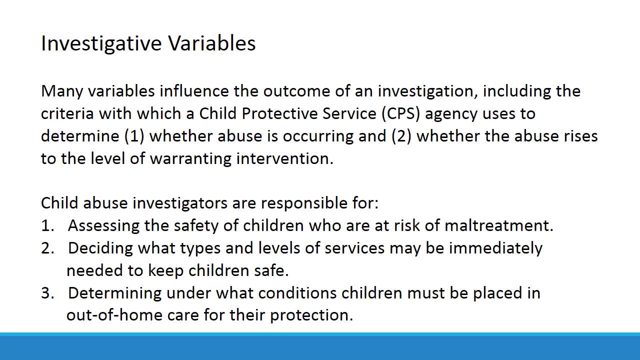 on forensic interviewing techniques that avoid any type of suggestive or leading questions. Many variables influence the outcome of an investigation, including the criteria with which a child protective service agency uses to determine, one, whether abuse is occurring and, two, whether the abuse rises to the level of warranting. 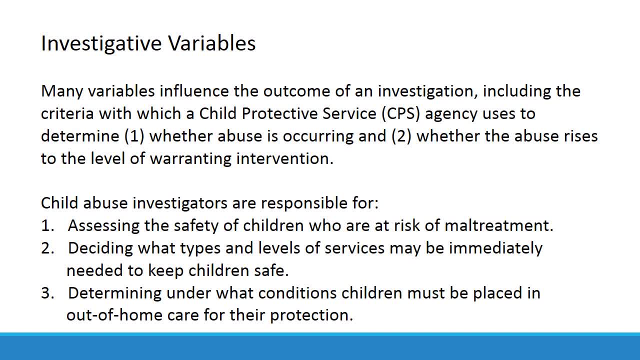 intervention. Child abuse investigators are responsible for: number one, assessing the safety of children who are at risk of maltreatment. number two, deciding what types and levels of services may be immediately needed to keep children safe. and number three, determining under what conditions children must be placed in The National Institute of Child Health and Human Development. 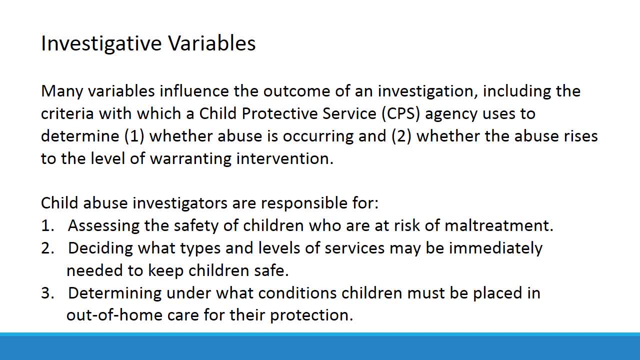 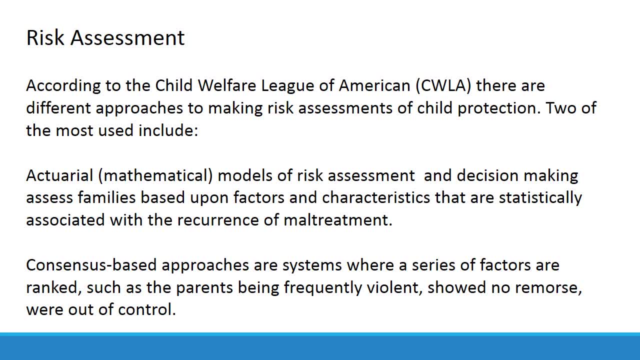 also influencesplant recommendations and uses the child welfare family's claims to assess child services's performance at risk. Each assessment now presented on the National Institute of Child Health and Human Developmentum will involved in região Intr " child welfare league of another. there are different approaches to making risk assessments of child 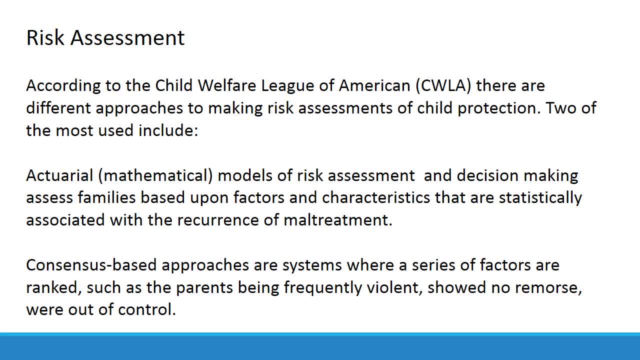 protection. Two of the most used include the actuarial or mathematical models of risk assessment and decision-making, which assess families based upon factors and characteristics that are statistically associated. we talked to a pianist earlier, an aspects of child, domestic, of maltreatment. So basically they're using the probability or the odds of something happening. 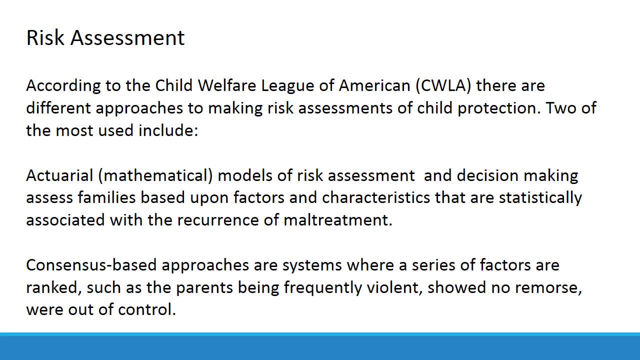 again. The second approach is consensus-based approaches, which are systems where a series of factors are ranked, such as the parents being frequently violent, showing no remorse, being out of control, And where these factors line up, will develop where the risk lies. 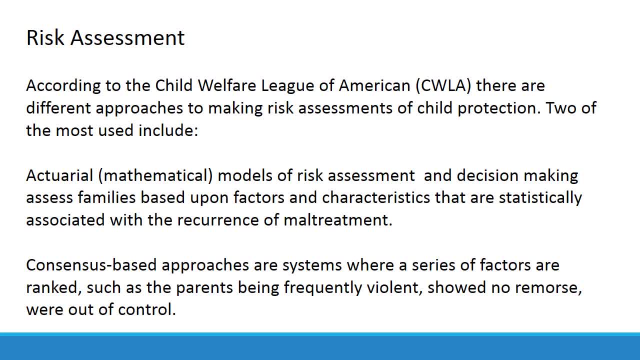 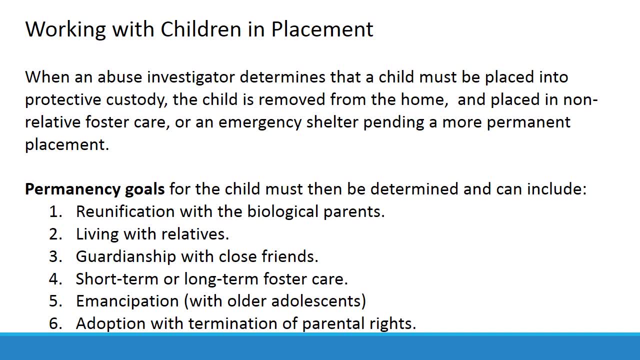 whether it being a high-risk or a low-risk scenario. When an abuse investigator determines that a child must be placed into protective custody, the child is removed from the home and placed in non-relative foster care or an emergency shelter pending a more permanent placement. Permanency goals for the child must then be. 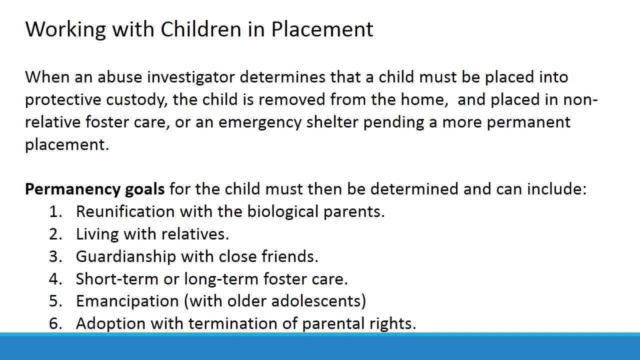 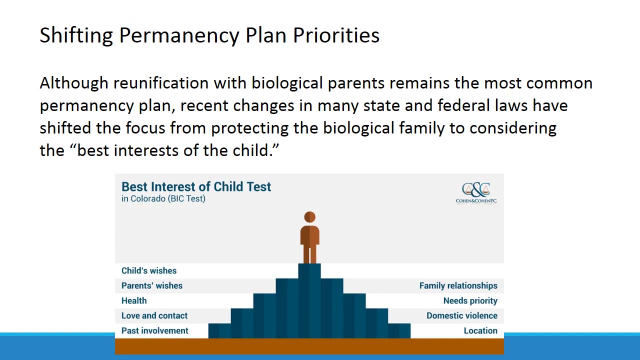 determined and can include reunification with the biological parent, living with relatives, guardianship with close friends, short-term or long-term foster care, emancipation with an older adolescent, maybe somebody who's 17,, and adoption with termination of parental rights, Shifting permanency plan priorities. So, although reunification 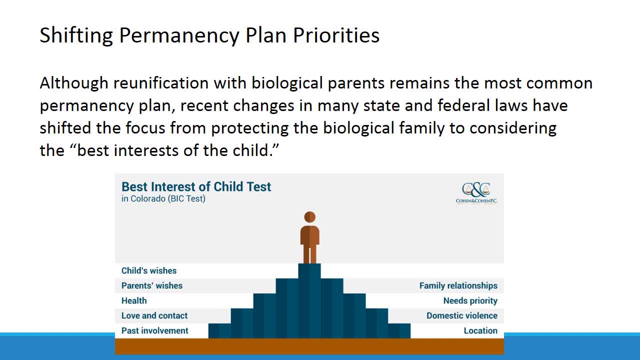 with biological parents remains the most common permanency plans. recent changes have been made in many state and federal laws that shift the focus from protecting the biological family to considering the best interests of the child, And here is a chart from Colorado that looks at these nine elements when deciding what. 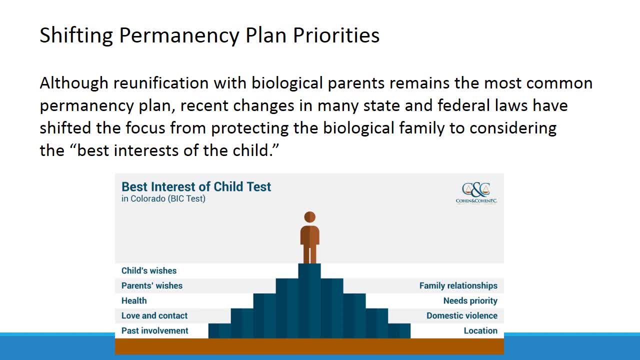 one should do with the child. So if the child has been living in a scenario where they've been maltreated and the parents have been living in a scenario where they've been mistreated and the parents have not pursued any remediation to repair their behavior, you have to look. 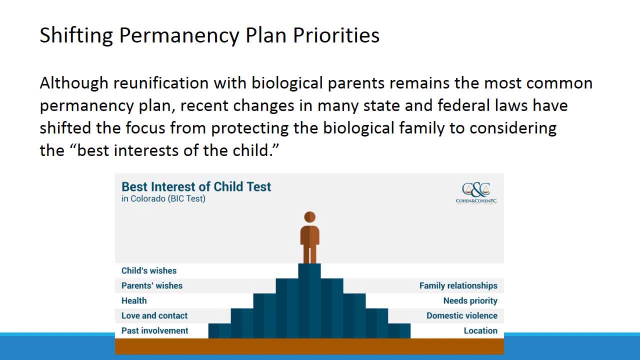 at other options, And the other options we have to look at involve these things where what is the priorities for the child? Maybe the best option is for him or her to live with a relative or friends of the child's relative Or, you know, live with parents of friends of the child. So there's a lot of issues. 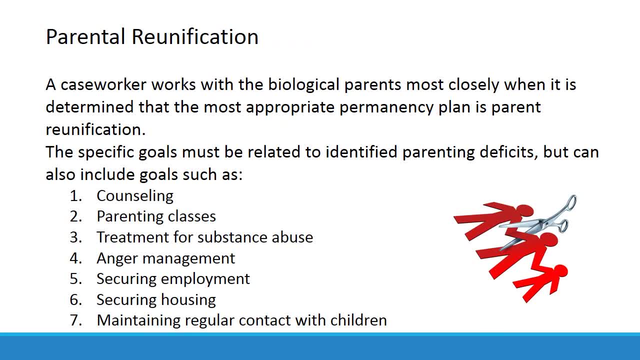 that may go on there. So let's talk about parental unification. A caseworker works with the biological parents most closely when it is determined that the most appropriate permanency plan is parental reunification. The specific goals must be related to identified parenting deficits. but can also include goals like parental rem Allegheny And for parental unification. the parents must choose the appropriate plan. in case of parental imlegtency, The parents must agree with the parent's decision to keep the parent in the parent position for the child. 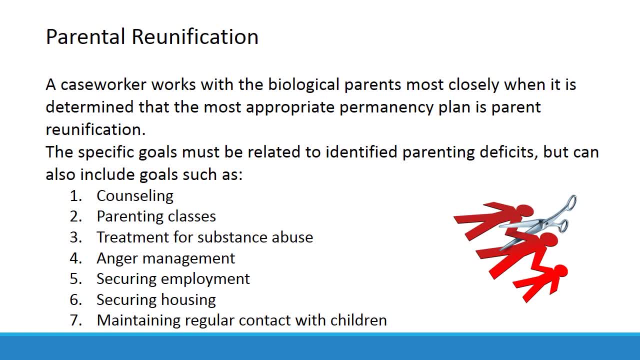 and the parents must agree with the parent's decision to keep the parent in the parent position for the child, such as counseling, parenting classes, treatment for substance abuse, anger management, securing employment, securing housing and maintaining regular contact with children. So, if a child is removed from a household because one or both parents has a substance abuse problem, in this particular regard, 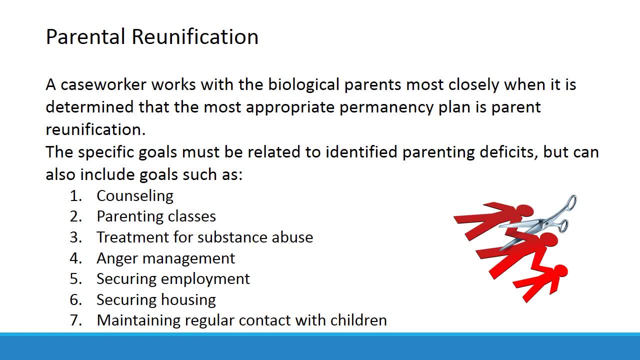 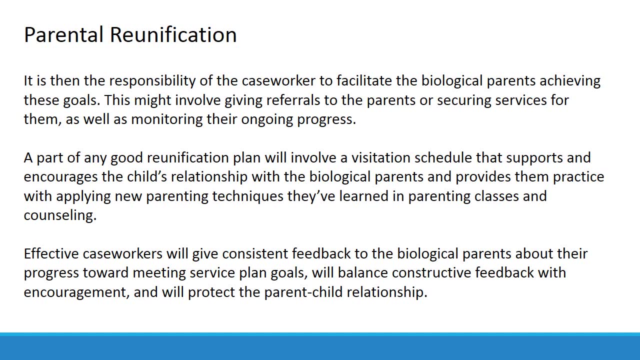 we're then going to be hoping or seeing that the parent goes through treatment so that the child can be reunited with their parent. It is then the responsibility of the caseworker to facilitate the biological parents achieving these goals. It doesn't mean that the parents are not responsible for their behavior. They have to do their part. 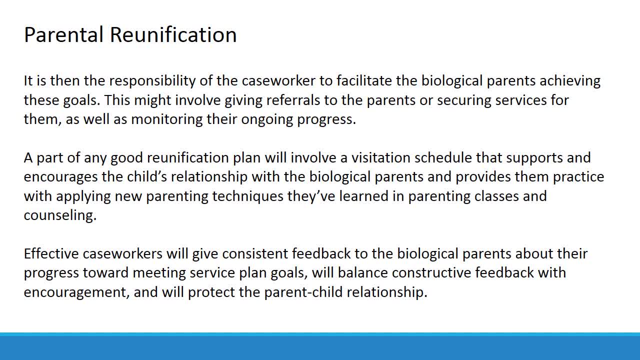 This might involve giving referrals to the patients or securing services, as well as monitoring their ongoing process. As part of any good reunification plan, it will involve a visitation schedule that supports and encourages the child's relationship with the biological parents and provides them with practice with applying new parenting techniques they've learned in parenting classes and counseling. 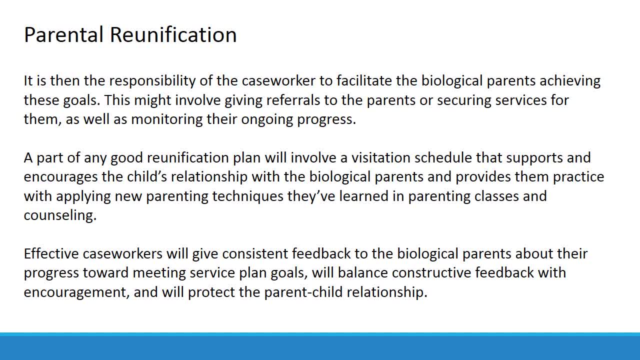 Effective caseworkers will give consistent feedback to the biological parents about their progress toward meeting the needs of their child. So if a child is removed from a household because one or both parents have a substance abuse problem, we're then hoping or seeing that the parent goes through treatment so that the child can be reunited with their parent. So if a child is removed from a household because one or both parents have a substance abuse problem, we're then hoping or seeing that the child goes through treatment so that the child can be reunited with their parents. This is one of many reasons that Пока ở các trường, tổ chức khôngatter g tha cteil m Startd these service plan goals. 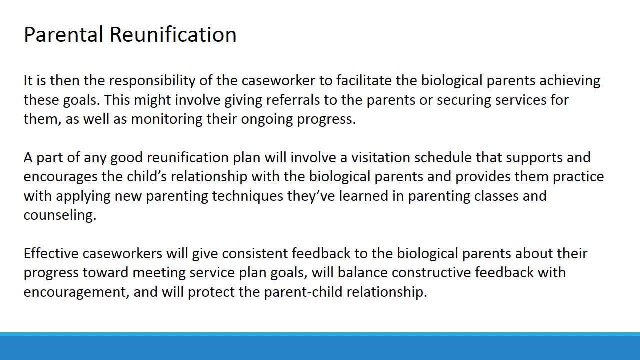 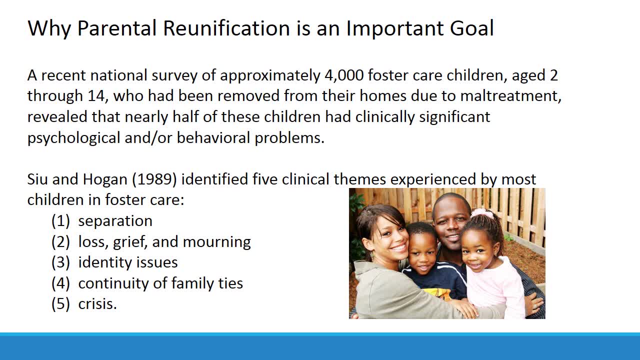 and will balance constructive feedback with encouragement and will protect the parent-child relationship. So why is parental reunification such an important goal? A national survey of approximately 4,000 foster care children aged 2 through 14 who have been removed from their homes due to maltreatment. 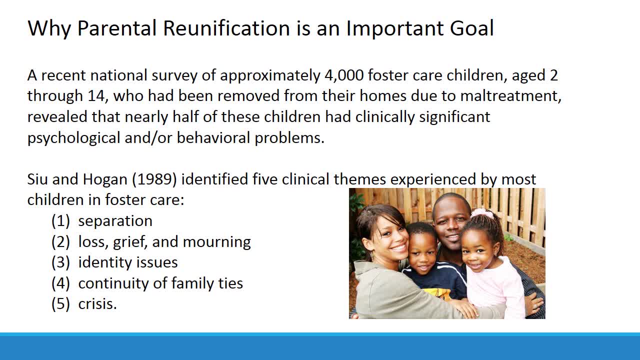 revealed that nearly half of these children had clinically significant psychological and or behavioral problems. Sue and Hogan, in a study in 1989, identified five clinical themes experienced by most children in foster care: Separation, loss, grief and mourning, identity issues, continuity of family ties and a feeling of being in crisis. 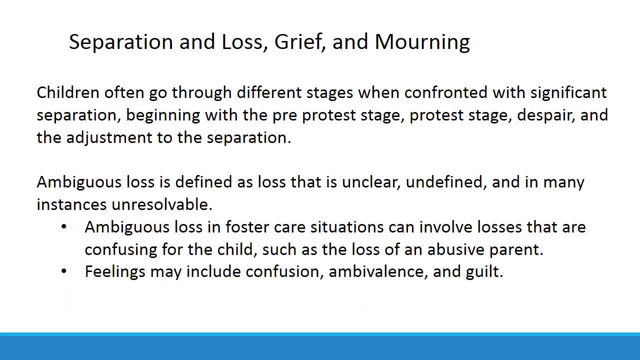 Children often go through different stages when confronted with significant separation, beginning with pre-protest stage, protest stage, despair and ultimately, the adjustment to the separation. It doesn't mean that they accept the separation, they eventually just adjust to it. The bigger issue is this idea of ambiguous loss, which is defined as loss that is unclear, undefined. 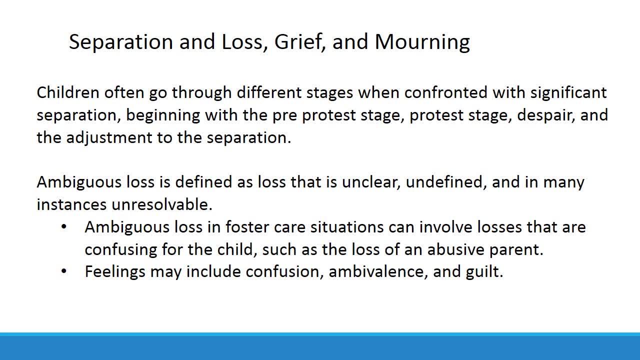 and in many instances it's not clear. As adults, we may understand why a child is removed from their home if mom and or dad have a substance abuse problem or a problem with their anger or abuse, but children who love mom and dad and don't understand that abuse is wrong. 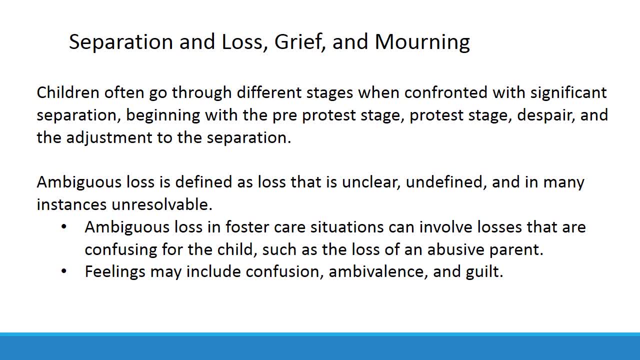 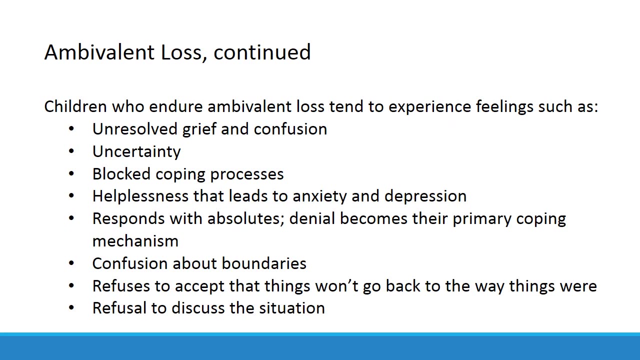 may feel this sense of loss, And this sense of loss is very confusing for the child And even though the parent is abusive or not supportive, they still feel confused, ambivalent and guilty to a certain extent. They also feel uncertainty, blocked coping processes, helplessness that leads to anxiety and depression. 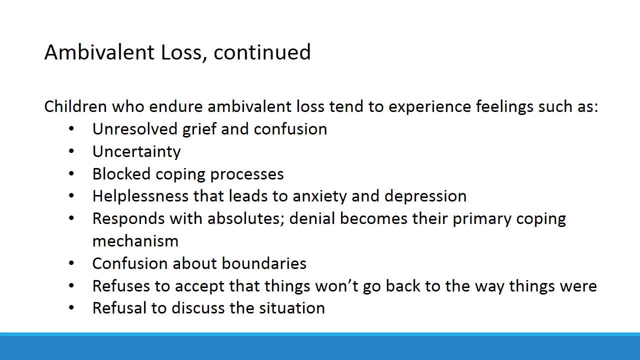 They respond with absolutes, And when they are denied, denial becomes their primary coping mechanism. They're confused about boundaries, they refuse to accept that things won't go back to the way things were, and they don't want to discuss the situation. 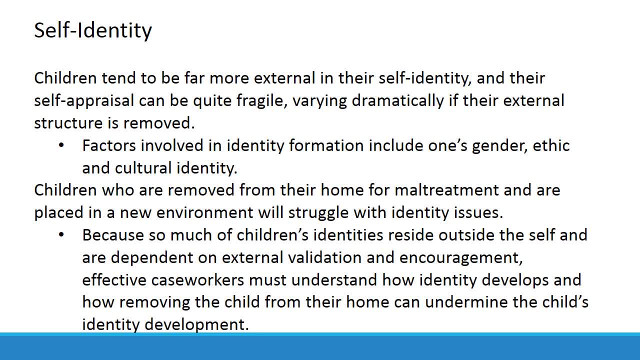 Additionally, self-identity becomes a big issue, especially as young people enter adolescence. Children tend to be far more external in their self-identity and their self-discovery And their self-appraisal can be quite fragile, varying dramatically if their external structure is removed. 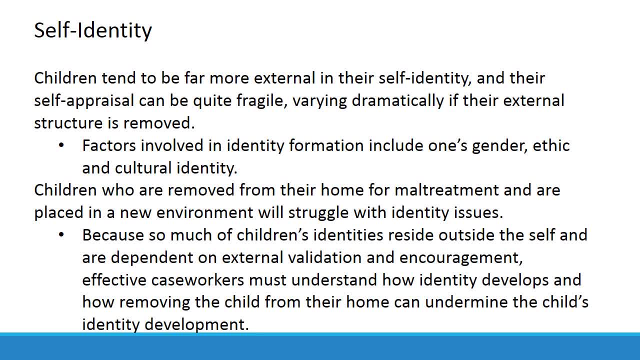 So take them away from what they identify as their identification as family, and those things undermine who they feel they are. So factors that are involved in identity formation include one's gender, ethnic and cultural identity. children who are removed from their home for maltreatment and are placed in a new environment will struggle with identity issues. 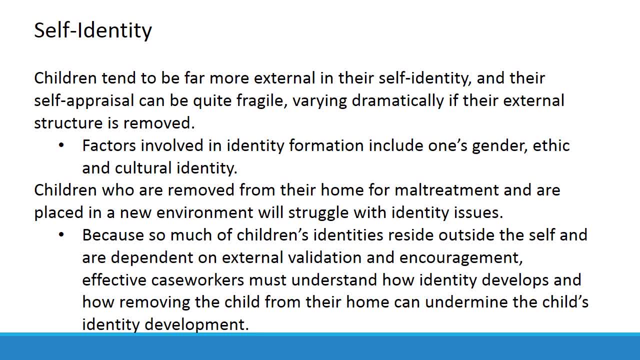 Because so much of children's identities reside outside the self and are dependent on external validation and encouragement. effective caseworkers must understand how identity develops and how removing the child from their home can undermine the child's identity development. So, if you think about adolescence, 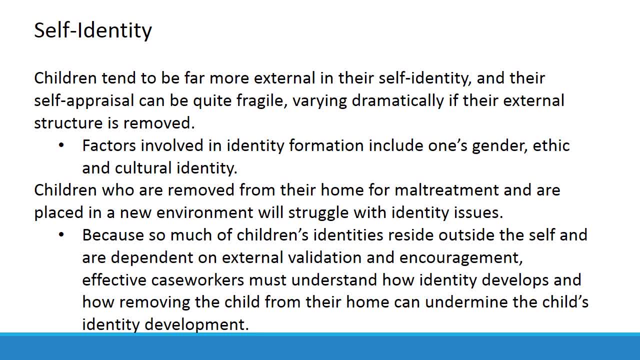 and you think about how in 7th grade, your average 12-13 year old might still be a kid and as they emerge through or evolve through their teen years, they may try different quote unquote identities. They might try playing sports. 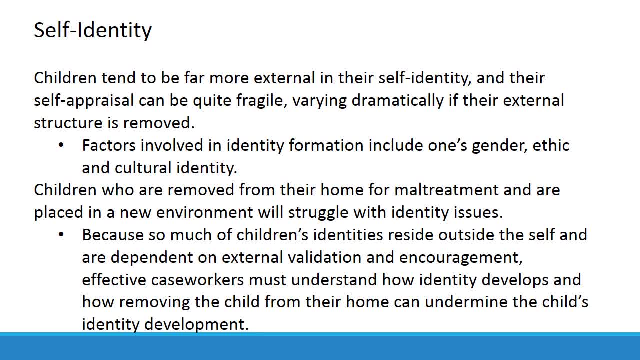 they might try being into theater, they might try singing, they might try acting, they might try any number of things, They might try any number of skills or different activities to find that activity that really connects with them And that's how they develop their sense of who they are. 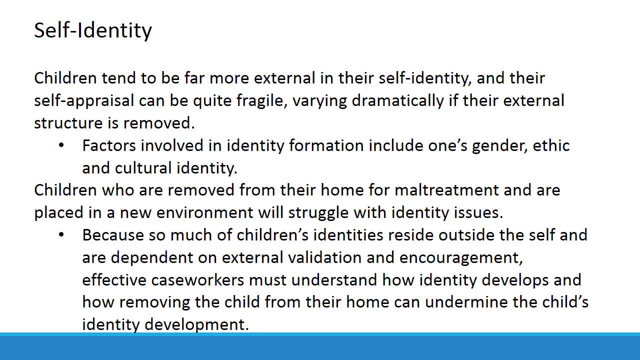 And part of that is based on where they come from. So if they don't know where they're coming from anymore, they automatically develop this sense of they don't know who they are on the inside, so they can't figure out who they are on the outside. 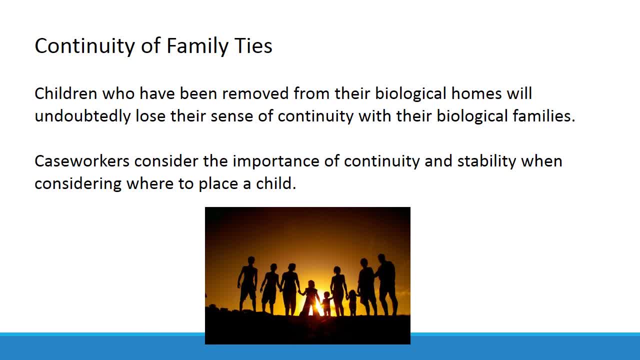 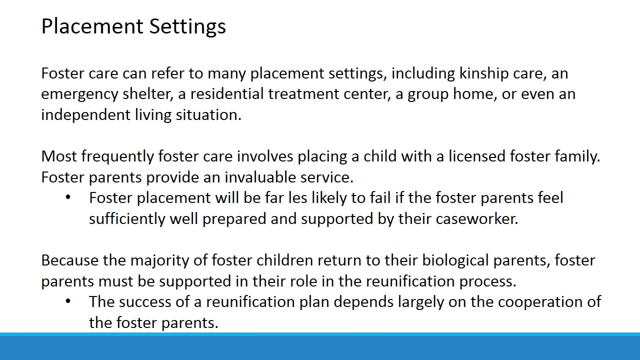 Children who have been removed from their biological homes will undoubtedly lose their sense of continuity with their biological families. Caseworkers consider the importance of continuity and stability when considering where to place a child. Foster care can refer to many placement settings, including kinship care. 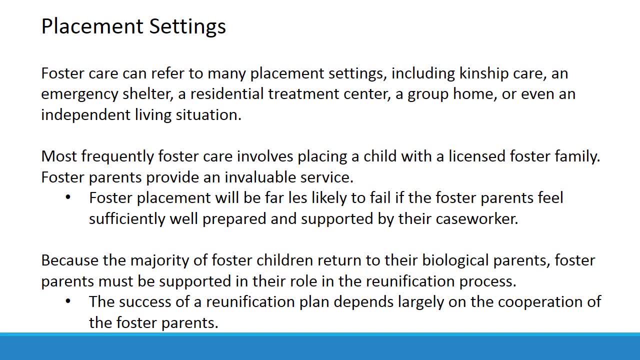 an emergency shelter, a residential treatment center, a group home or even an independent living situation. Most frequently, foster care involves placing a child with a licensed foster family. Foster parents provide an invaluable service. Foster placement will be far less likely to fail. 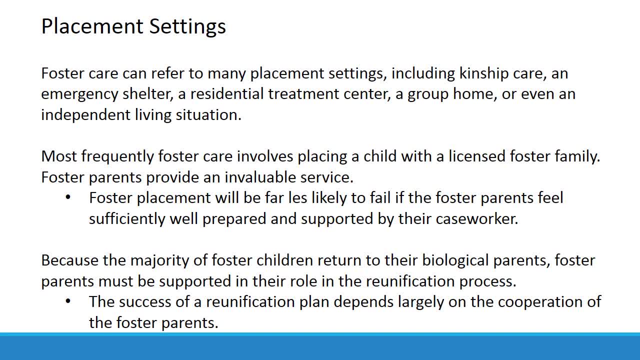 if the foster parents feel sufficiently well prepared and supported by their caseworker. Because the majority of foster children return to their biological parents, foster parents must be supported in their role in the reunification process. The success of a reunification plan depends largely on the cooperation of the foster parents. 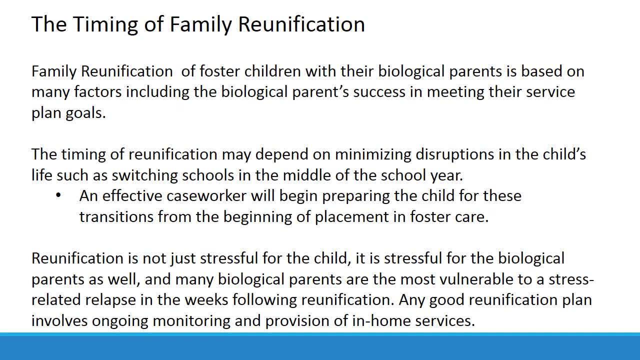 Family reunification of foster children with their biological parents is based on many factors, including the biological parent's success in meeting their service plan goals. So if the family reunification is based on the parents completing a drug rehabilitation program and the parents do not complete that program, 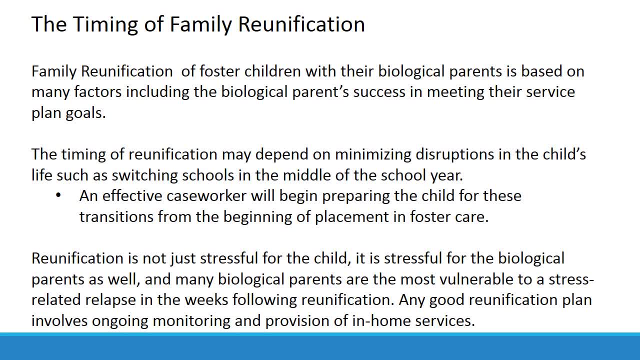 well, that in and of itself will halt the family reunification, But the timing otherwise is oftentimes based around how to minimize the disruptions in the child's life, such as switching schools. in the middle of the school year, An effective caseworker will begin preparing the child. 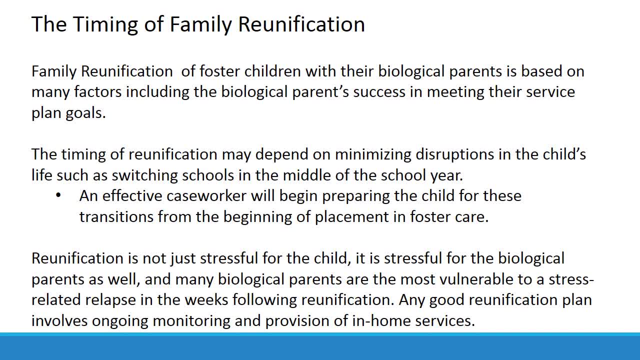 for these transitions from the beginning of placement in foster care. Reunification is not just stressful for the child, It is stressful for the biological parents as well, and many biological parents are the most vulnerable to stress-related relapses in the weeks following reunification. 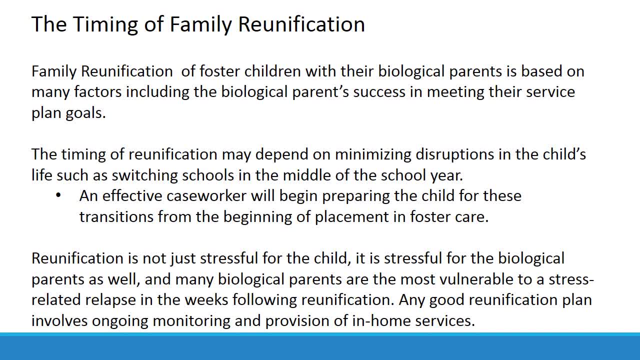 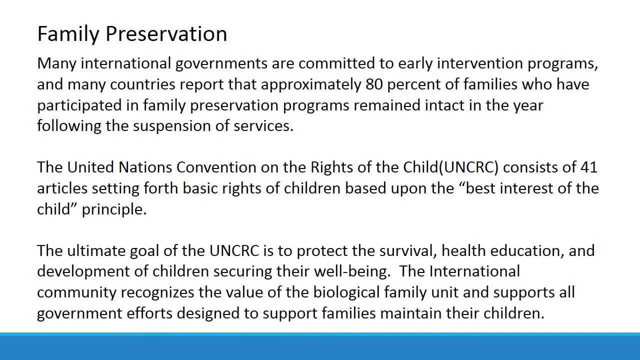 Any good reunification plan involves an ongoing monitoring and provision of in-home services. Many international governments are committed to early intervention programs and many countries report that approximately 80% of families who have participated in family preservation programs remained intact in the year following the suspension of services. 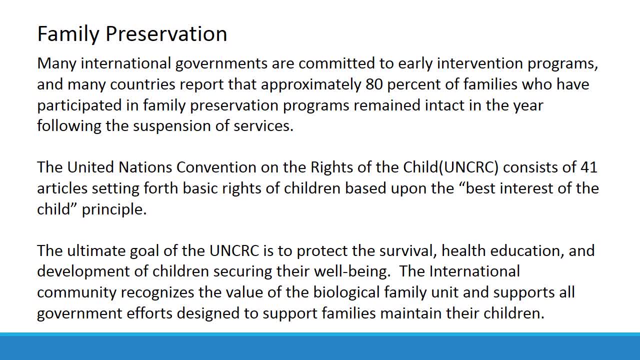 The United Nations Convention on the Rights of the Child consists of 41 articles setting forth basic rights of children based upon the best interests of the child. The ultimate goal of the UNCRC is to protect the survival, health, education and development of children. 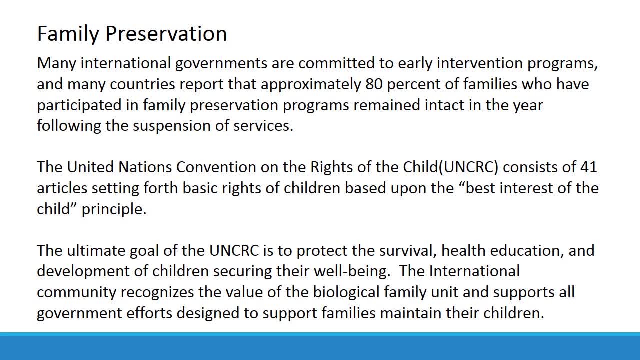 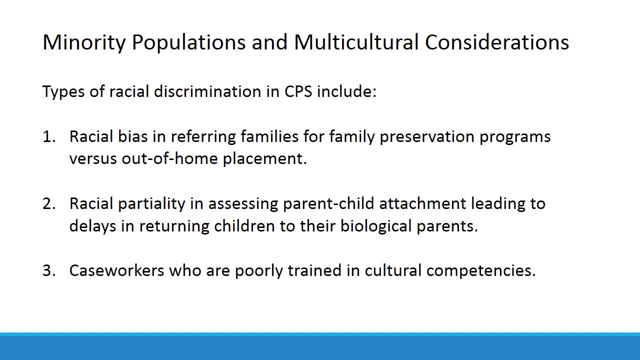 securing their well-being. The international community recognizes the value of the biological family unit and supports all government efforts designed to support families maintain their children. So let's talk about minority populations and minority children. The United Nations Convention on the Rights of the Child talks about minority populations and multicultural considerations. 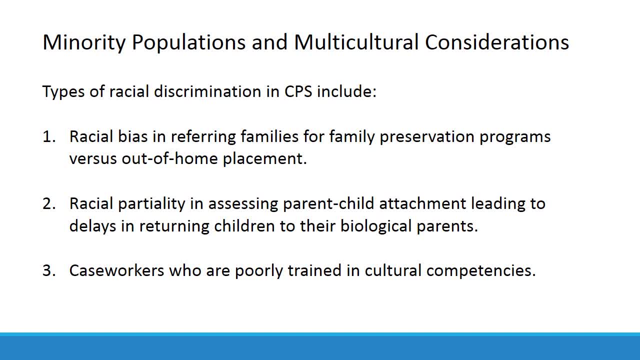 Types of racial discrimination that one sees in child protective services include racial bias in referring families for family preservation programs versus out-of-home placement, racial partiality in assessing parent-child attachment, leading to delays in returning children to their biological parents, and number three caseworkers who are poorly trained in cultural competencies. 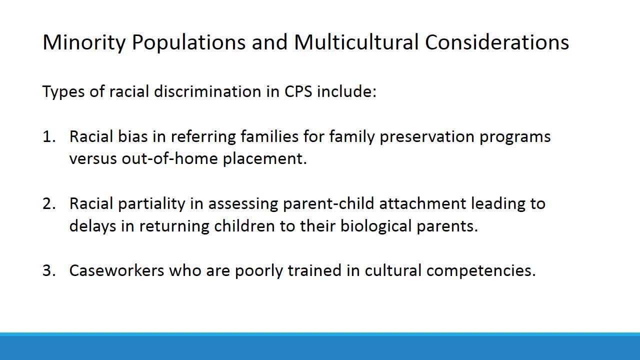 So what this basically means is that most people who get into the social work or behavioral health industry or career field are people who are not necessarily your prejudicial discriminatory types. But we all have these unconscious or subconscious biases, Or we're just not trained sufficiently to understand. 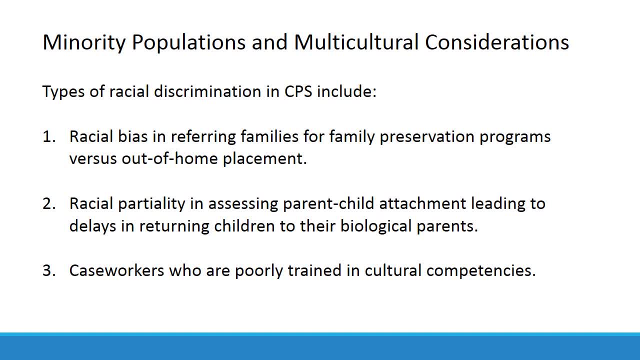 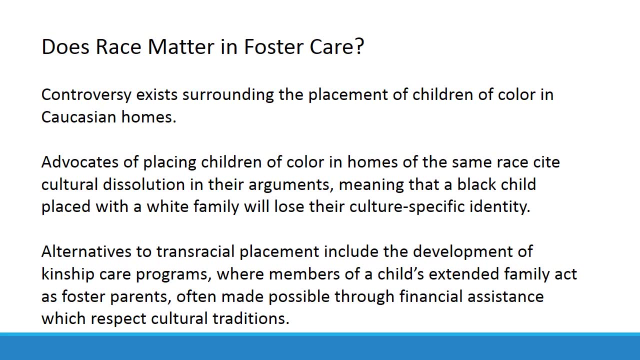 the historical aspects of race and bias in our particular society And, as a consequence, there are issues that we still deal with today. So does race matter in foster care? Controversy exists surrounding the placement of children of color in Caucasian homes. Advocates of placing children of color in homes of the same race. 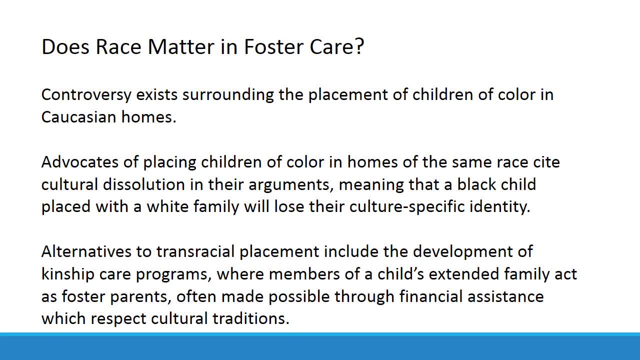 cite the cultural dissolution as their argument, meaning that a black child placed with a white family will lose their culture-specific identity. So the idea here is that there are very specific cultural aspects to being African American in the United States that a white family would not understand. 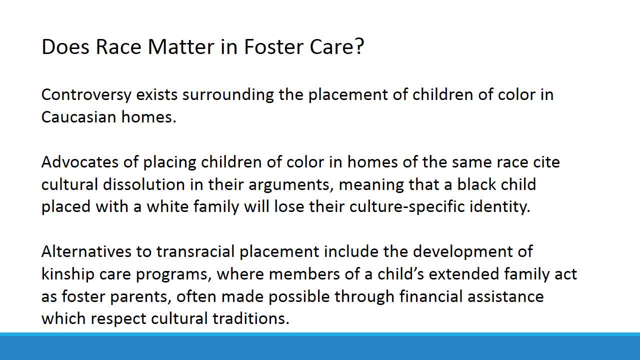 And that is absolutely true. The other side of that is: should a black child have to wait for a foster family for an extra week, two weeks, three weeks if there are no African American foster families available? So it's not an easy solution. 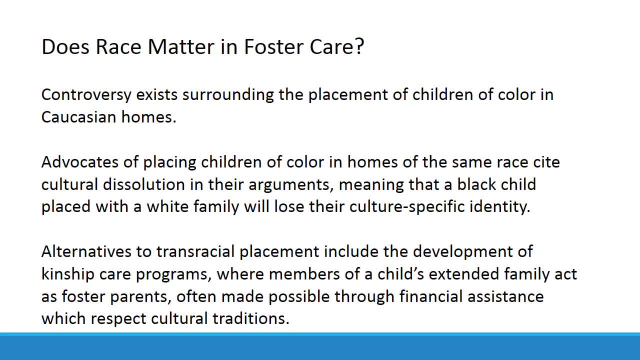 Alternatives to transracial placement include the development of kinship care programs, meaning someone in the family or someone close to the family become foster parents, where members of the child's extended family act as foster parents, often made possible through financial assistance which respect the cultural traditions. 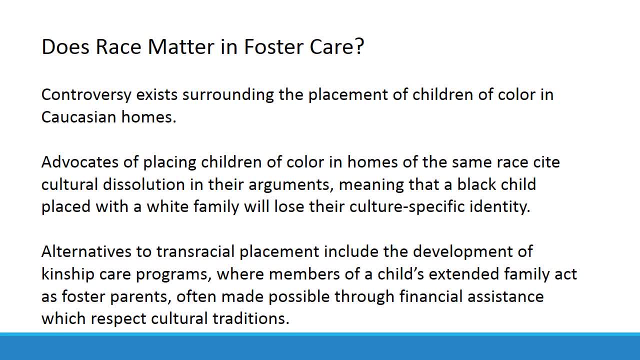 Now, this is not always possible, but there are alternatives being developed to try and help this. And again, this is a controversial thought process and it is understandable, but it's also something that there's no easy answers, Because if somebody needs love and support and help, 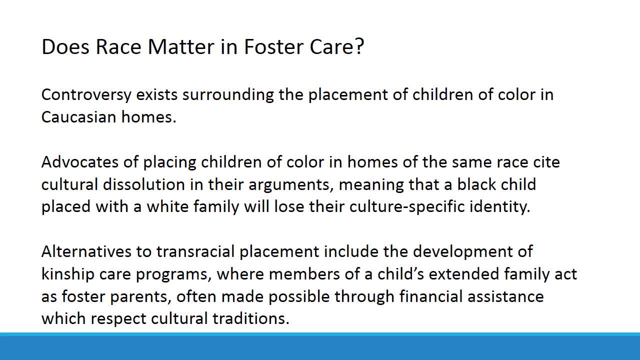 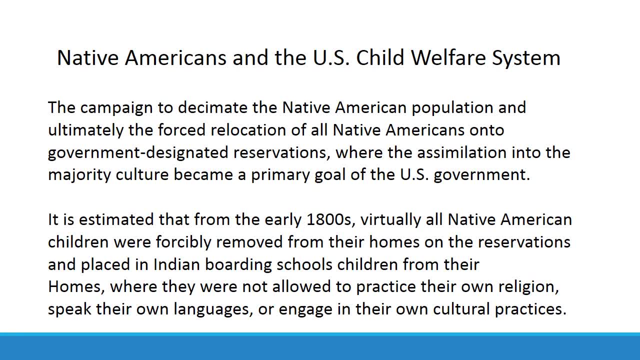 it doesn't matter to the child as much as to society who's giving it to them. So let's talk about the Native Americans and the United States child welfare system, And this is an example of why it's important to understand cultural history, Because not everyone has had positive experiences with the government. 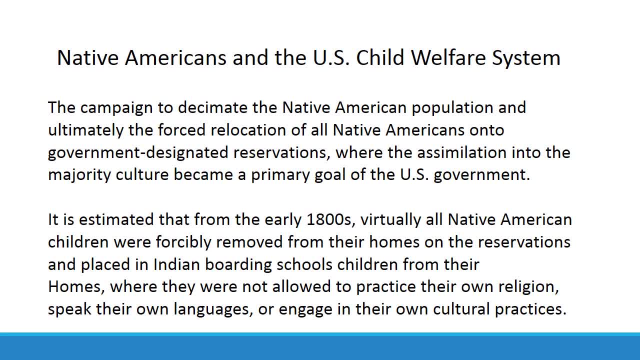 The campaign to decimate the Native American population and ultimately force relocation of all Native Americans onto government-designated reservations, where the assimilation into the majority culture became the primary goal of the United States government. It is estimated that from the early 1980s, 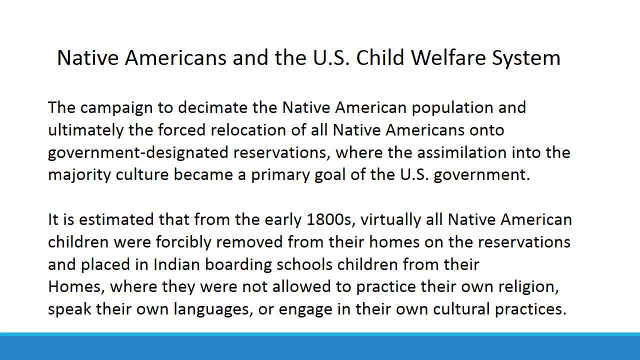 to the early 1800s, virtually all Native American children were forcibly removed from their homes on the reservations and placed in Indian boarding schools, taking the children from their homes, where they were not allowed to practice their own religion. they were not allowed to speak their own languages. 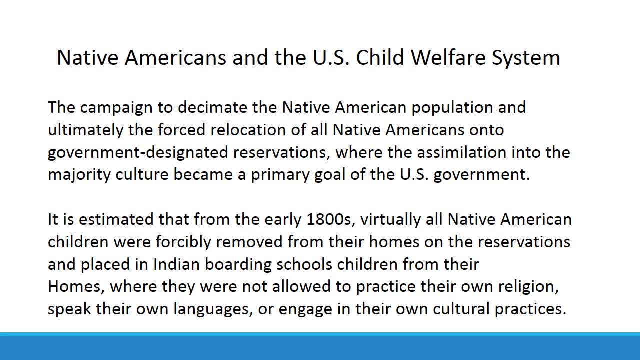 or engage in any of their own cultural practices. So you have a system that American history kind of glosses over, And this is not to beat up American history at all. This is, in fact, an important part of why behavioral health specialists and human services people need to understand. 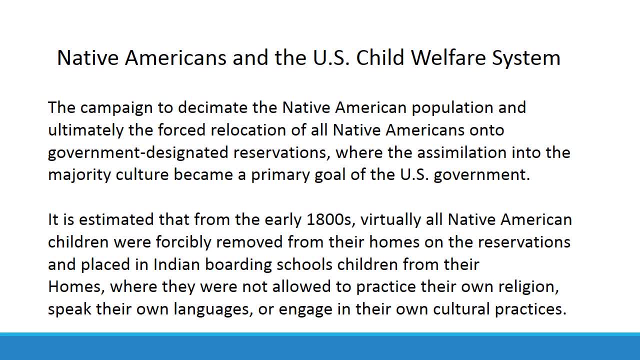 why there is distrust against the government, Because they did this, And Adolf Hitler wrote about this- about the fact that the United States government did a great job decimating the Native Americans And that's what he was trying to do with the Jews. I mean, that's a pretty scary thought to think about. 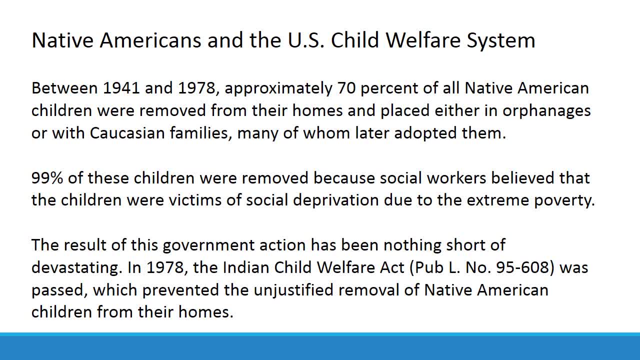 Between 1941 and 1978, approximately 70% of all Native American children were removed from their homes and placed either in orphanages or with Caucasian families, many of whom later adopted them. 99% of these children were removed because social workers believed. 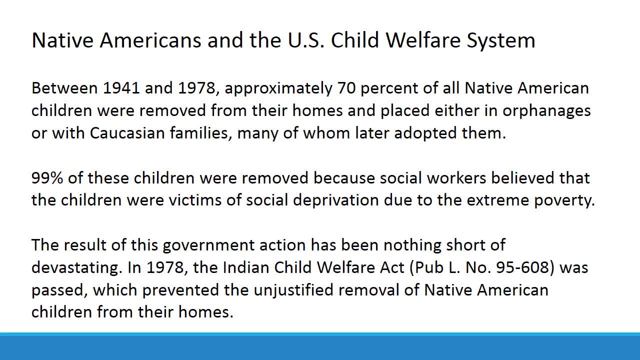 that these children were victims of social deprivation due to extreme poverty. And why were they living in extreme poverty? Because the reservations were basically ghettos for Native Americans. The result of this government action has been nothing short of devastating In 1978,. 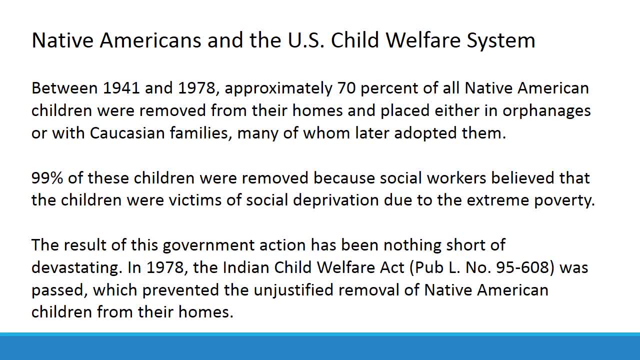 the Indian Child Welfare Act was passed, which prevented the unjustified removal of Native American children from their homes, And you know, to think about how recent this is is what is truly stunning. So we have to keep in mind again that, as much as we want to do the right thing, 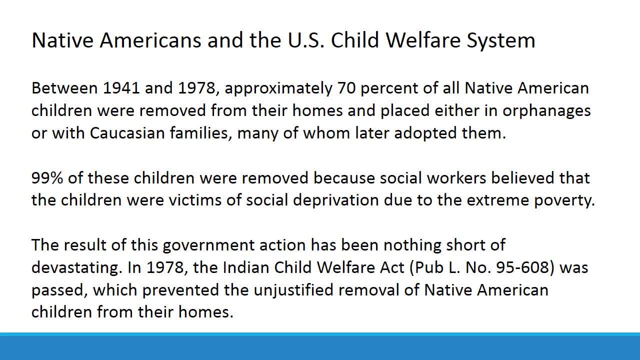 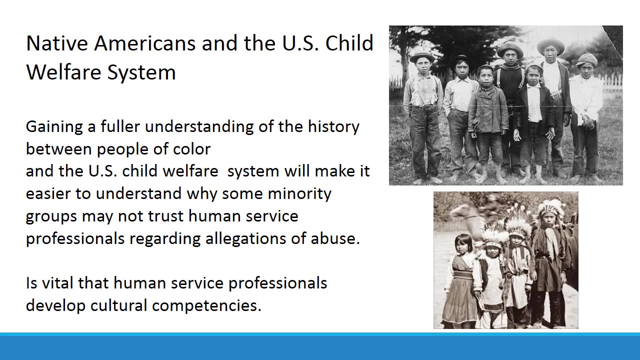 we have to remember that there's a historical precedent that we're oftentimes fighting against because historically we didn't always do the right thing. Gaining a fuller understanding of the history between people of color and the US child welfare system will make it easier to understand.